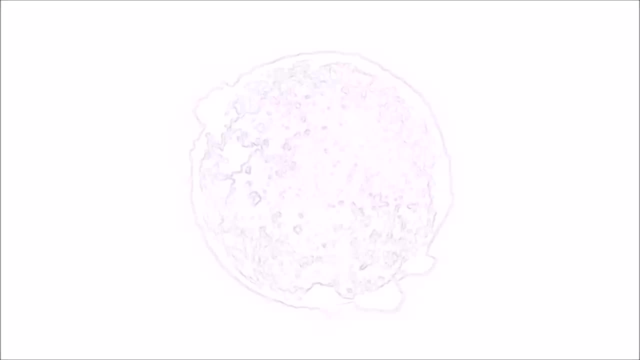 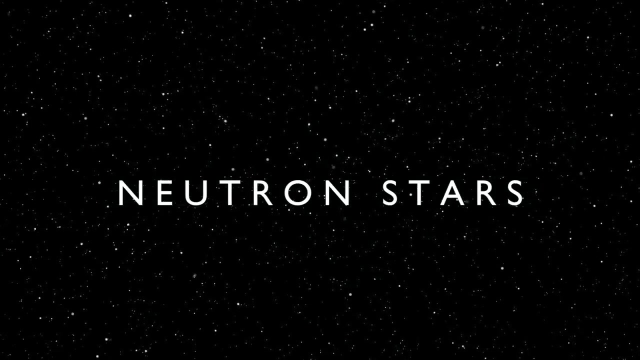 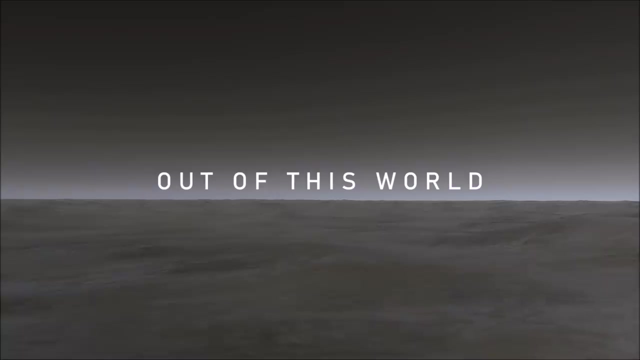 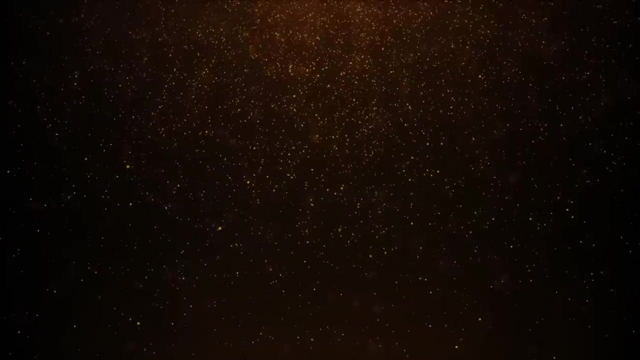 tortured matter so dense and compressed that the effects are out of this world quite literally. These dense graveyard star cores are known as neutron stars, and their types, properties and statistics are all absolutely mind numbing. In order to understand what a neutron star is, you must first understand what a neutron 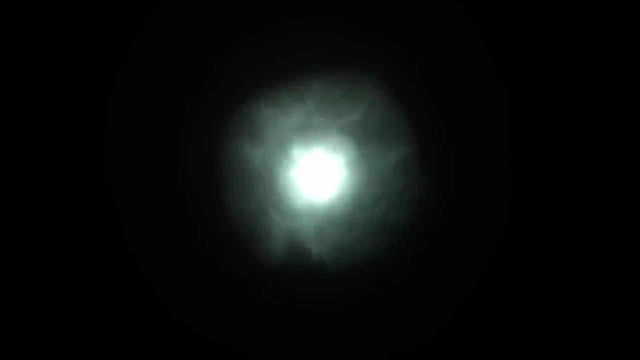 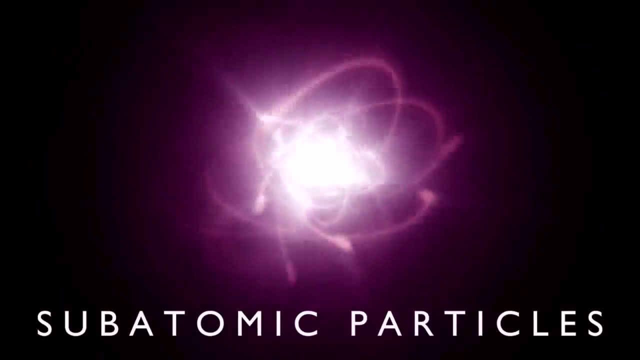 is Everything in the universe besides energy is composed of atoms, the tiny fundamental building blocks of creation, And they themselves are made up of tiny components called subatomic particles, which come in three varieties: Protons, which have a positive electrical 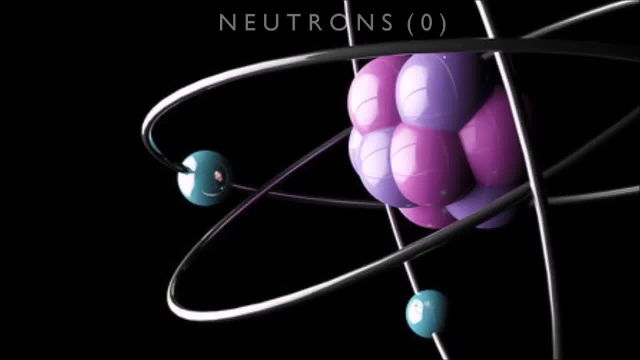 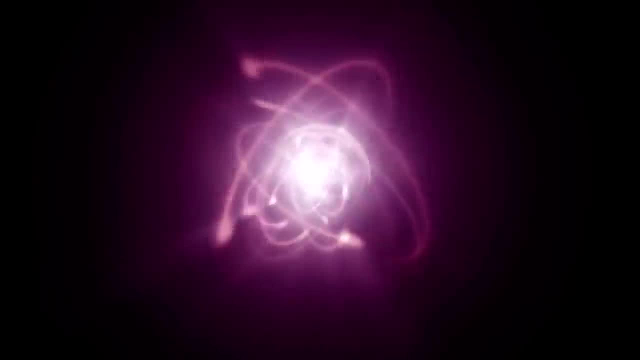 charge, electrons, which have a negative electrical charge, and finally, neutrons, subatomic particles with no net electrical charge. Protons and neutrons make up the nucleus of an atom and the number of each is the same in most elements. So, with that in mind, how does it relate? 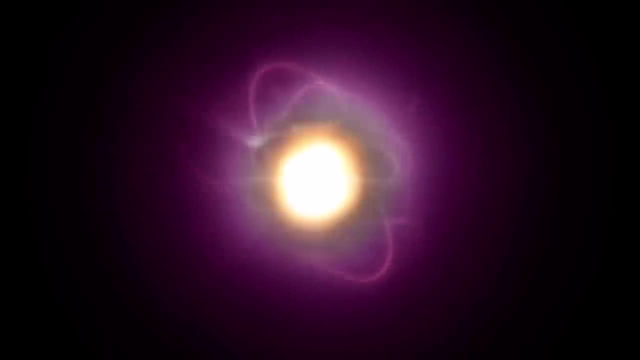 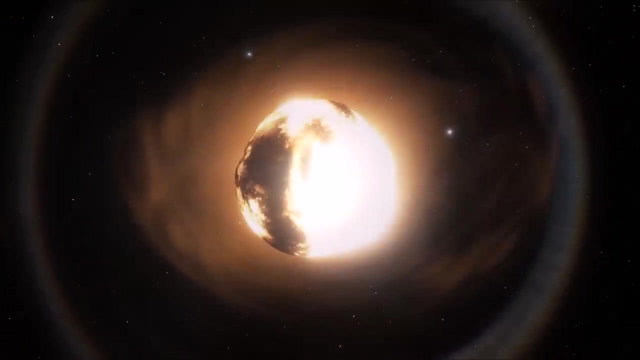 to dead stars. Well, a neutron star is formed when a massive star, between 10 times and 29 times the mass of our sun, reaches the end of its life and explodes. At this point, heavier elements in the core begin fusing iron, Because iron has no energy to give. fusion is no longer generating outward pressure from within the star and there is suddenly nothing to stop the star collapsing under the weight of its own gravity. The outer layers collapse inwards rapidly with nothing to counter them, and when they reach the iron core, this matter forces the interior into. 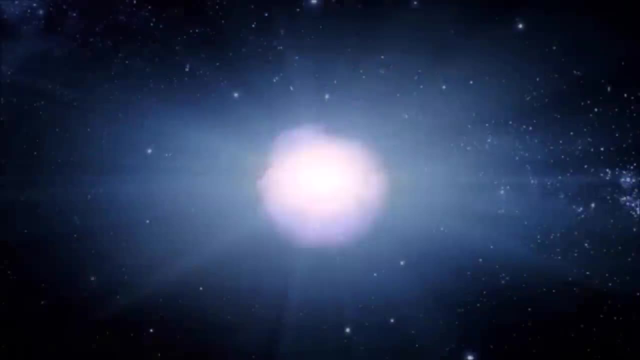 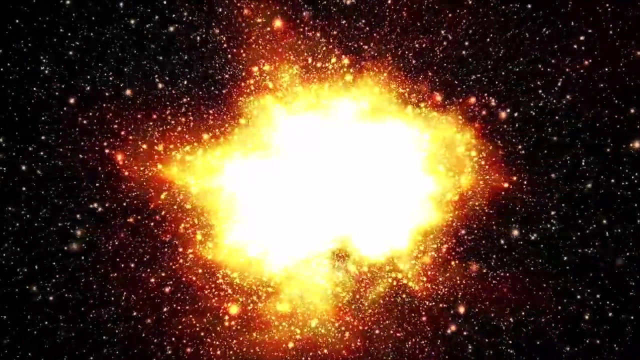 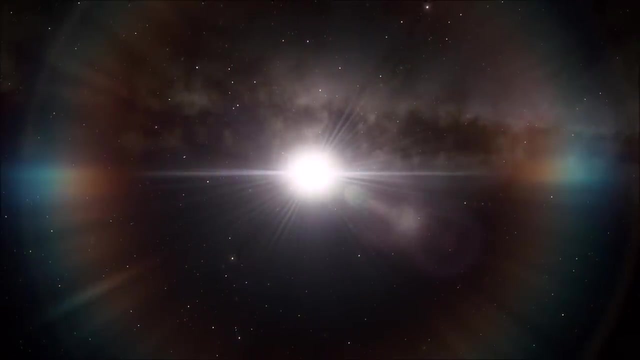 a much smaller space before essentially bouncing off the core and exploding in a violent supernova explosion. These outer layers collapse fast, at 25% the speed of light. in fact, This is so fast that particularly massive stars keep on collapsing indefinitely into a singularity, creating a black hole. A neutron star is formed by 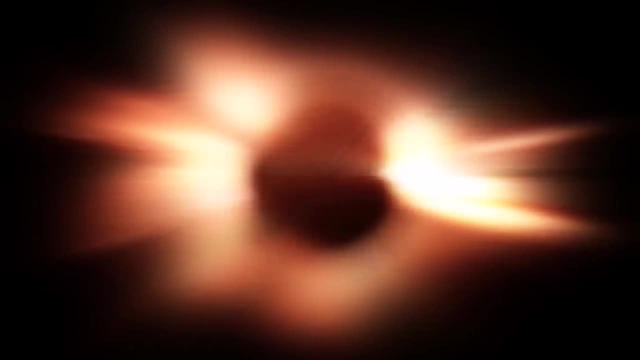 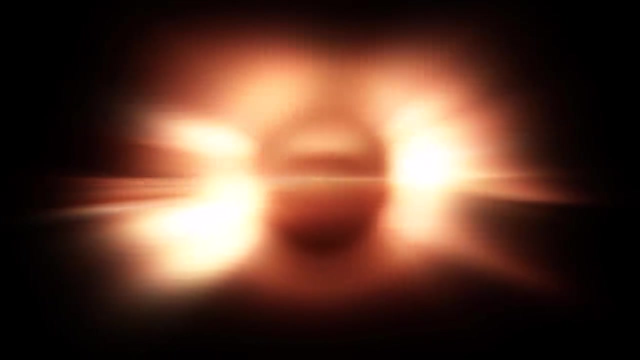 the level of massive star below star cores that are less than about 4-5 times the mass of the sun. In this case, the core is not massive enough to collapse indefinitely, but what remains of the collapsed matter is minuscule in size. 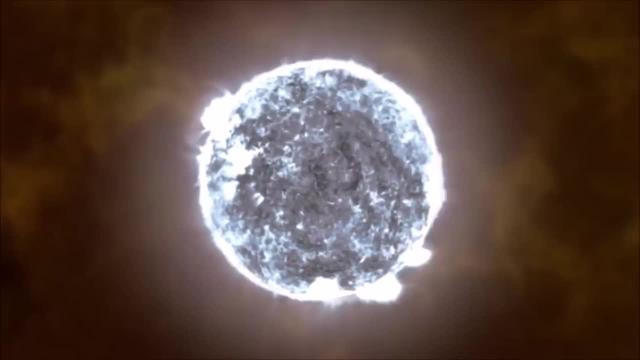 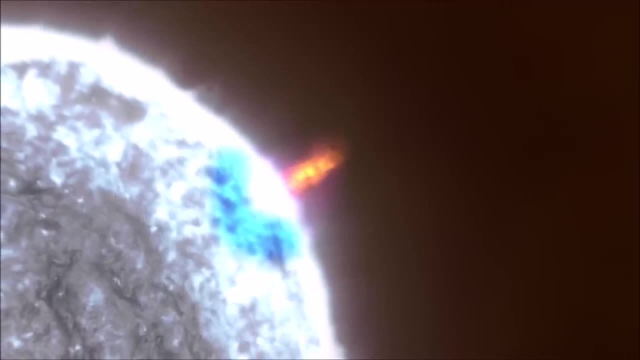 compared to its previous form. A star once hundreds of times larger than the sun collapses into an object the size of a city, making it among the densest objects in the universe. The reason they are called neutron stars is because the density and pressure on the interior 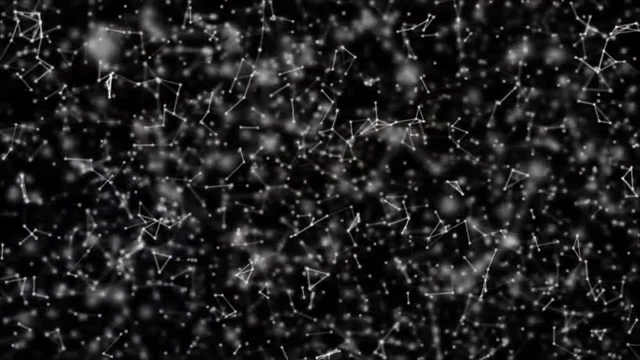 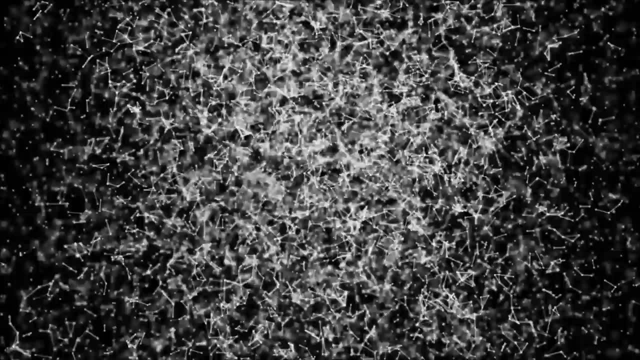 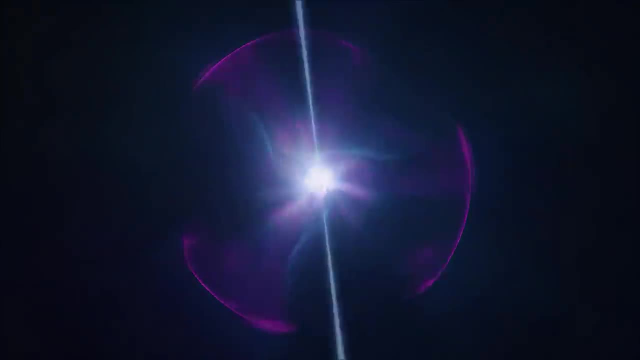 is so great that the protons and electrons of the atoms within start to be crushed into one another, generating long chains of strong neutron-rich material under conditions similar to those of the nucleus of an atom. Neutron stars are essentially giant atomic nuclei. These dense dead stars have extremely 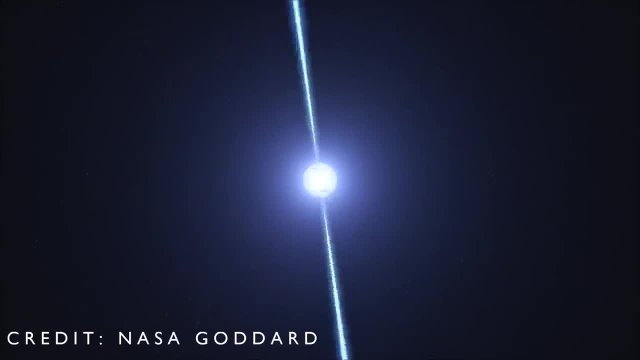 strong gravitational influences and magnetic fields. The chain reaction from the supernova explosion often causes the newly formed neutron star to spin incredibly quickly, with some known to rotate up to 40,000 times per minute, a speed which begins to deteriorate over time. 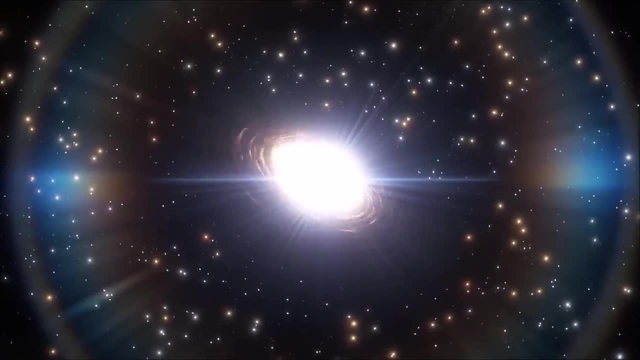 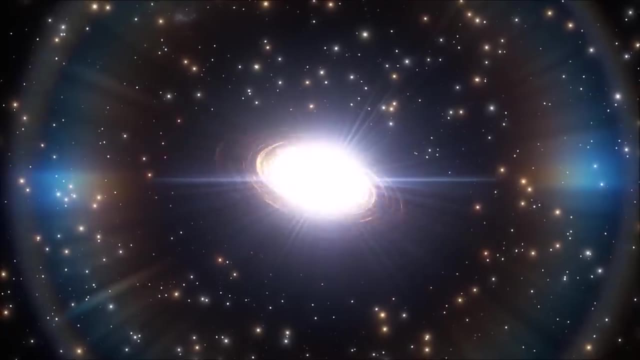 It wasn't until the 1960s that we were able to confirm the existence of these unthinkably dense objects, but scientists have been speculating on them for several decades. For example, after some 30 years or so, in the time leading up to their discovery In December 1933, just 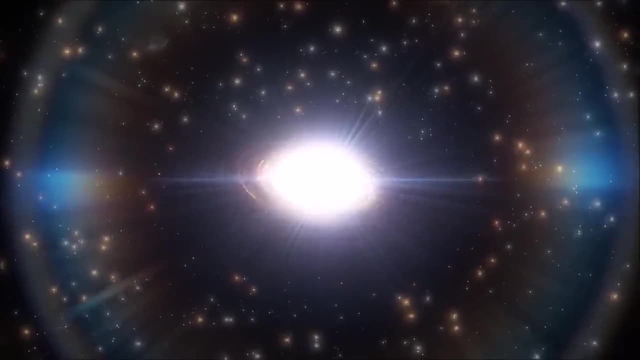 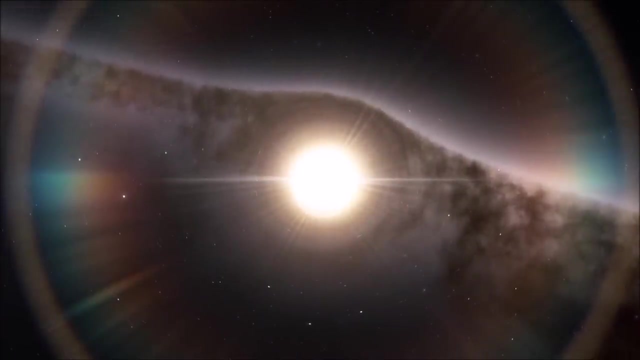 two years after the discovery of the neutron astrophysicists Walter Bade and Fritz Ficke proposed that supernova explosions could cause stars to turn into much denser, more closely packed bodies as a result of the explosion. A plausible theory, but at the time we were 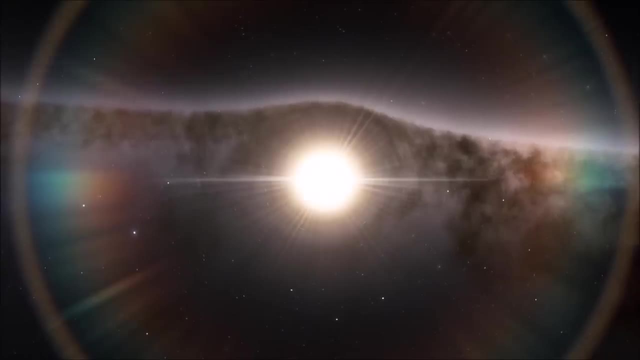 sure we'd never be able to detect such an object, even if they did exist, as they would simply be too small to be observed from the Earth. But moving into the 1960s, we were able to see that the neutron stars were actually. 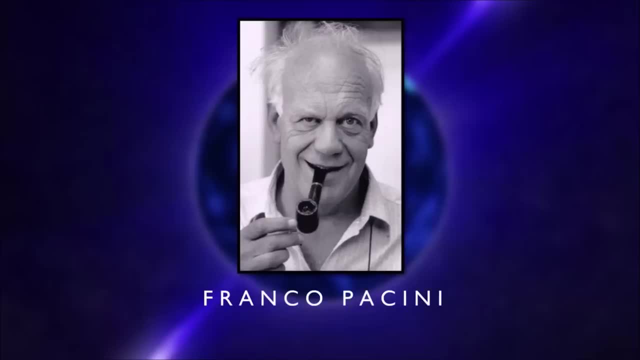 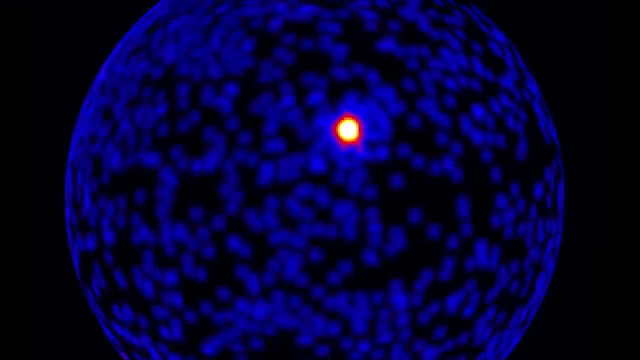 a source of radio brightness. In the 1960s, astronomer Franco Persini noted that if stars generated strong magnetic fields, then the electromagnetic radiation this would emit should be detectable from the Earth. And sure enough, in 1965, astronomers Anthony Hewish, 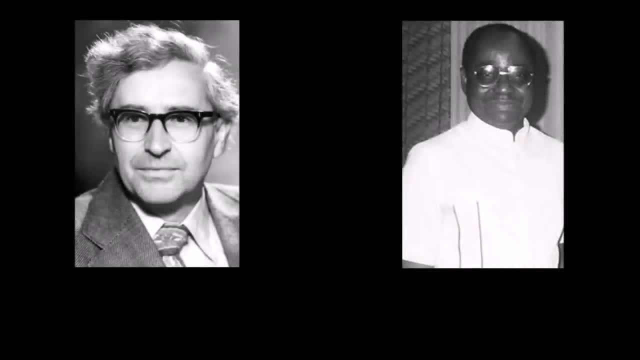 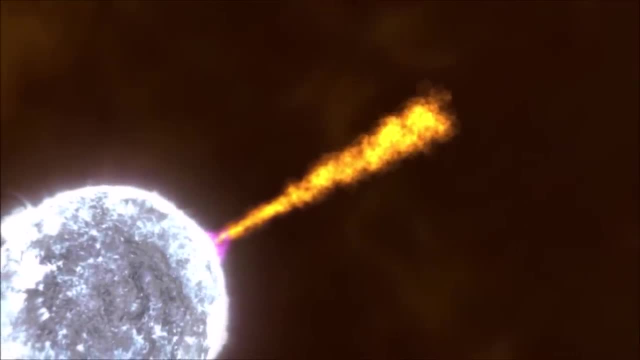 and Samuel Okoye discovered a source of radio brightness in the nearby Crab Nebula. This anomaly turned out to be the product of a rapidly rotating neutron star, and so we were able to conclude on the existence of these terrifying post-production stars. And then 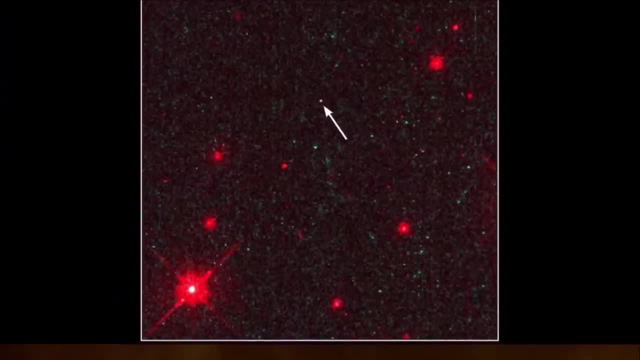 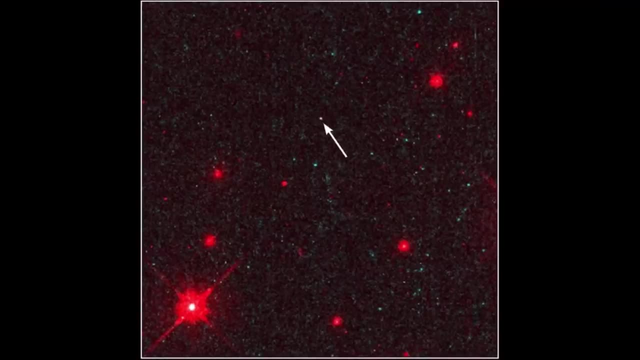 in 1997, we did in fact see a neutron star through visible light. What you see here is an actual photograph of a neutron star of a similar mass to our sun, which was discovered in 1992.. The achievement of observing a neutron star 400 light years away in visible light is not 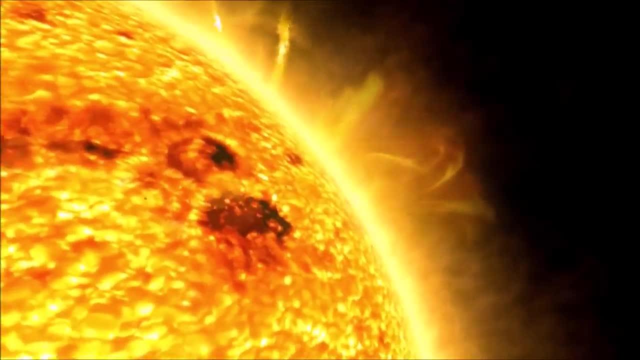 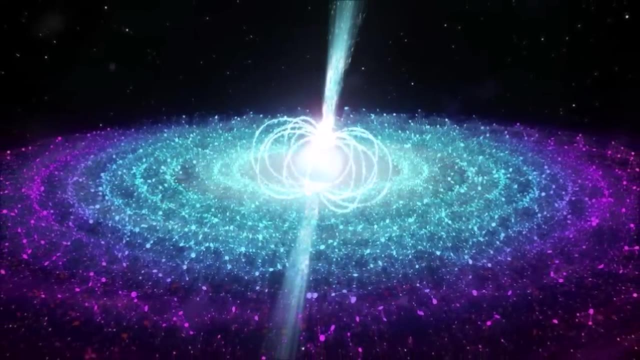 to be understated. Whereas stars are millions of kilometers in diameter and radiate light, most neutron stars are merely about 20km in diameter, or just 12 miles. One of the largest we've discovered to date is probably the most charging neutron star of our entire history. 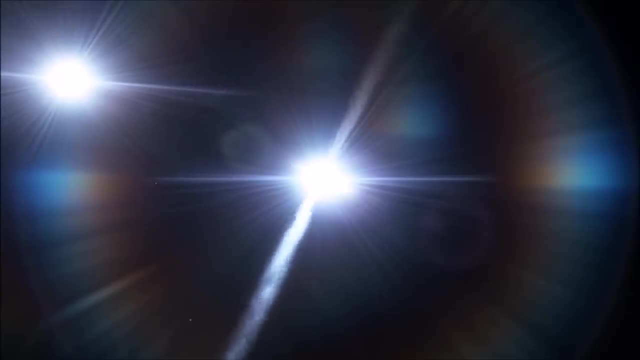 These stars are quite large. They must be at least 1.6m in diameter. They're not very large and in the end they can hold up to two cake blocks, and they could be connected to PSR J0348,, a neutron star in the constellation of Taurus with an estimated mass of about 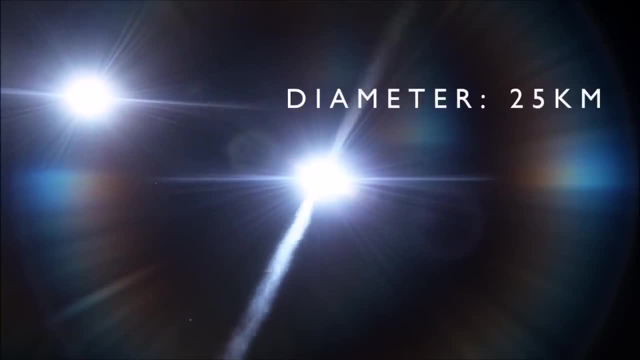 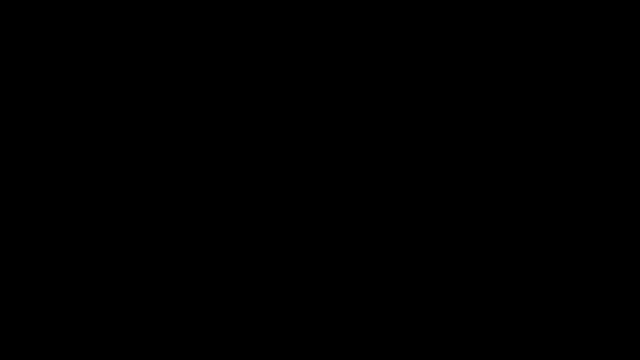 twice that of our Sun, packed into an object just 25 kilometres wide, making it smaller than the inner ring roads of the City of London, but huge for a neutron star, Although saying that size doesn't actually correlate to more mass within neutron stars, In fact more. 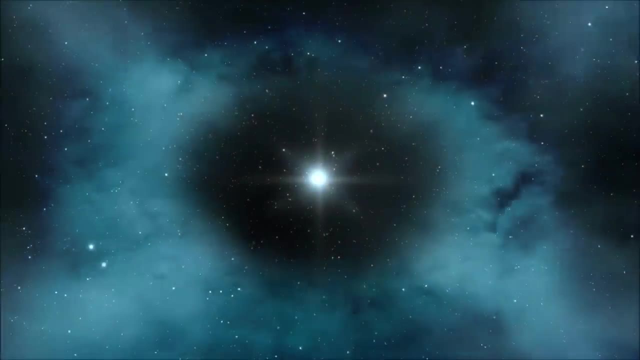 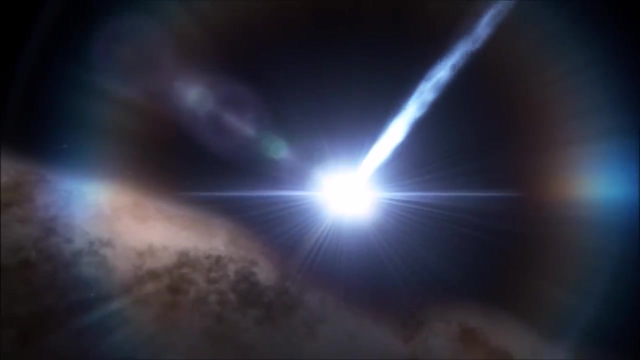 massive neutron stars are actually smaller, as their mass compacts more densely than in lighter neutron stars. Regardless of how big or small they are, this size-mass ratio gives them their incredible densities, so much so that a single teaspoon of neutron star matter. 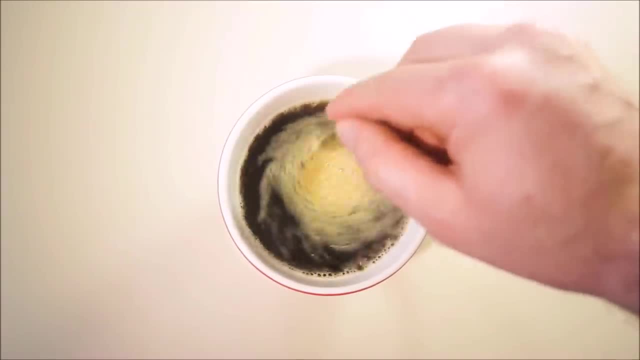 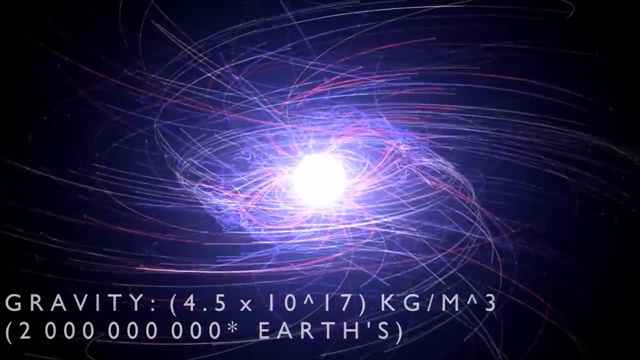 would weigh hundreds of millions of tonnes here on Earth. This incredibly compact concentration of mass means that the gravity of a neutron star is around 2 billion times greater than on the Earth And while not as dense as black holes, this gravity is still enough to bend. 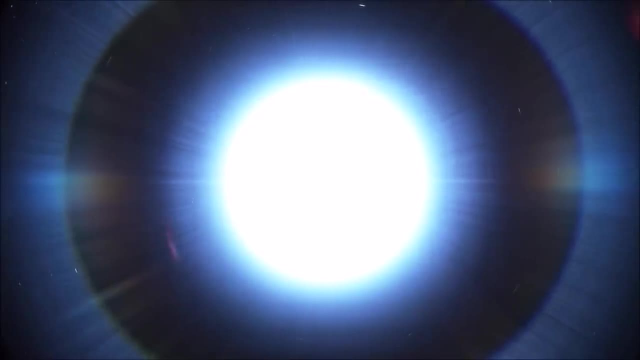 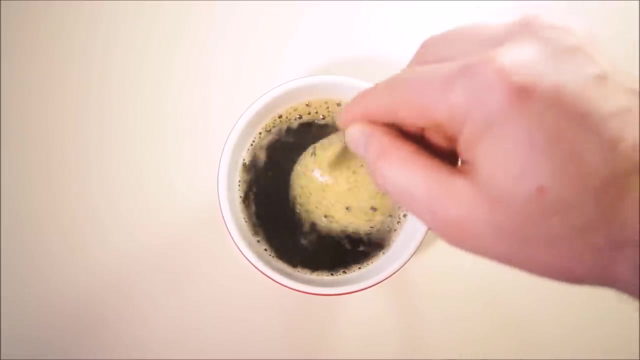 and warp the radiation and light being emitted around it, causing a gravitational lensing effect. In fact, sticking with our teaspoon of neutron star material, if you were able to drop it to the ground from shoulder height, the spoon would be travelling at well over 20,000 kilometres. 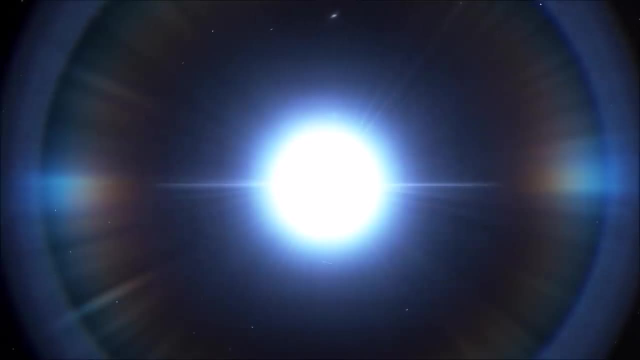 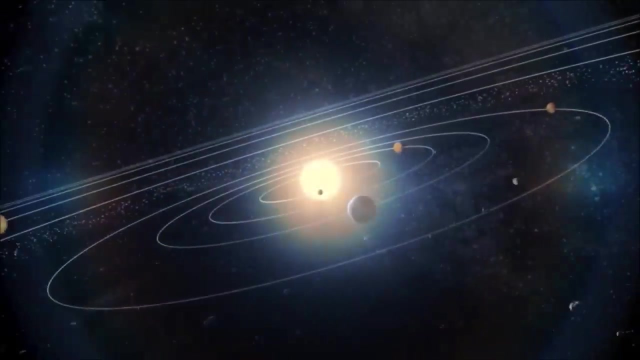 per hour before it collided with the ground. Our ideas on the nature of these stars is based on models, but it is possible to infer some details of a neutron star's structure by studying living stars such as the Sun. This process is known as astroseismology. 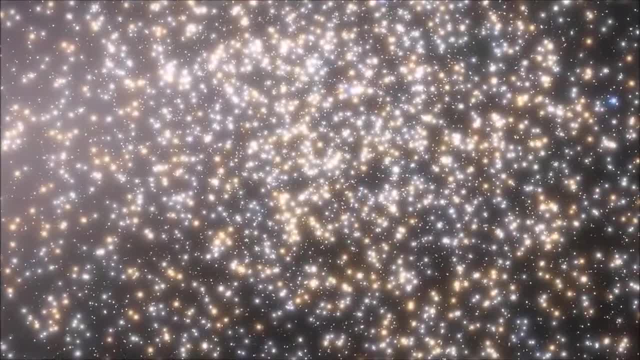 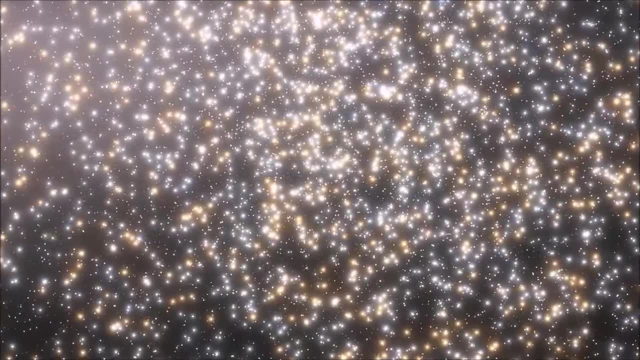 and it can reveal the inner structure of neutron stars by analysing the spectra of star os oscillations. This is what gives us our insight into the real jaw-dropping numbers associated with these cocoons. The surface or crust of the neutron star is an extremely hard 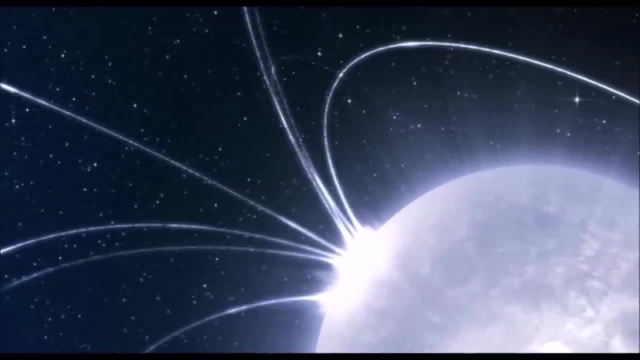 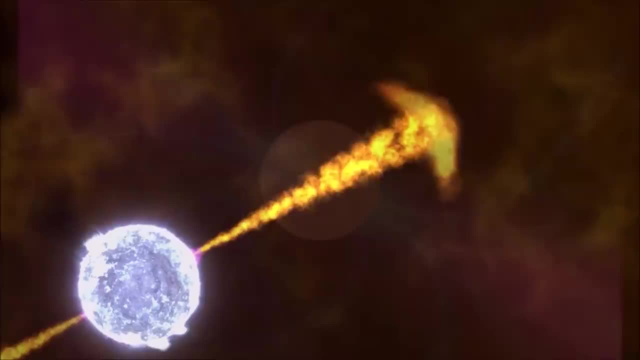 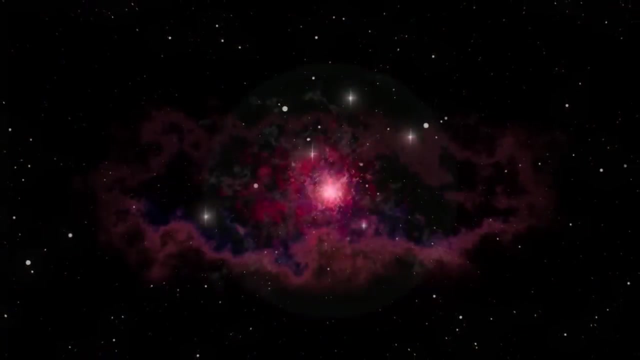 outer layer, whose surface temperature can reach up to 1 million degrees kelvin. This crust gives the neutron star a miniature landscape. It can have mountains, but these mountains can only ever hope to reach a few millimetres high. The extreme outer layer is made mostly of iron left over from the supernova, and this 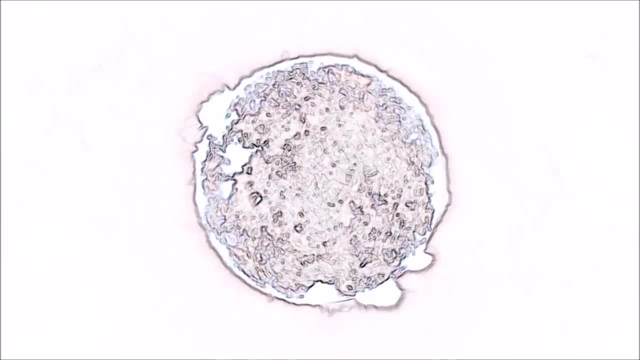 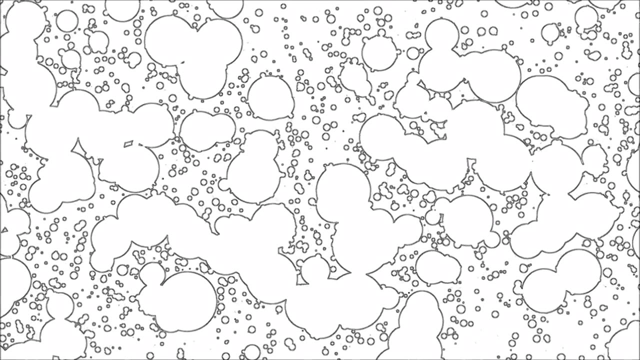 iron is so compressed that it keeps the neutron star in the atmosphere for a long time. This iron keeps the internal components sealed below the crust under unthinkable pressure. Under these conditions, atomic nuclei are crushed together in long strings of matter, trivially named nuclear pasta. Barely anything can breach this material. it is among the 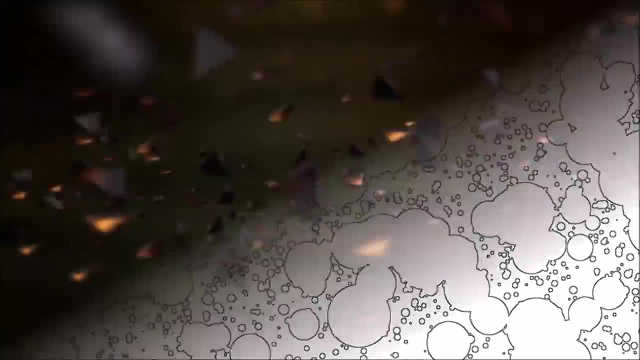 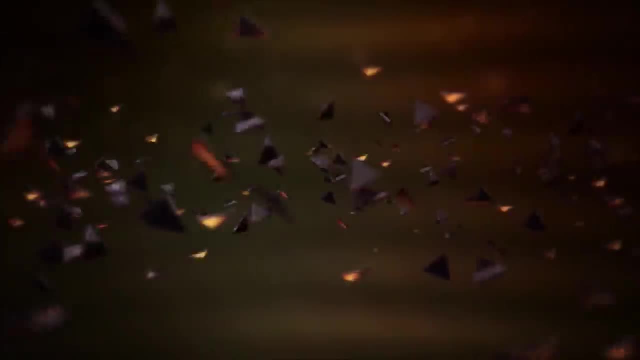 strongest and most tightly packed matter in the universe. As we move downwards towards the core, we start to become a bit less sure. We aren't sure what effect this much pressure, this deep into the core, would have on matter. However, we do note that it is able to keep. 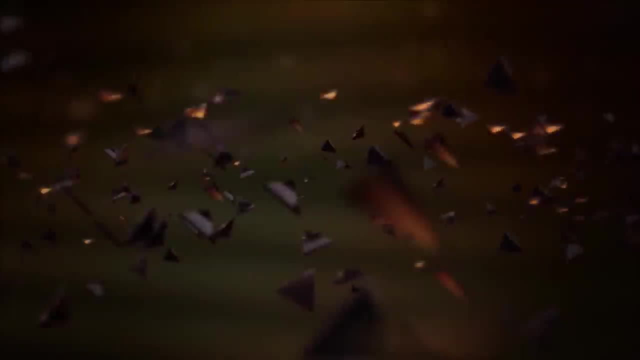 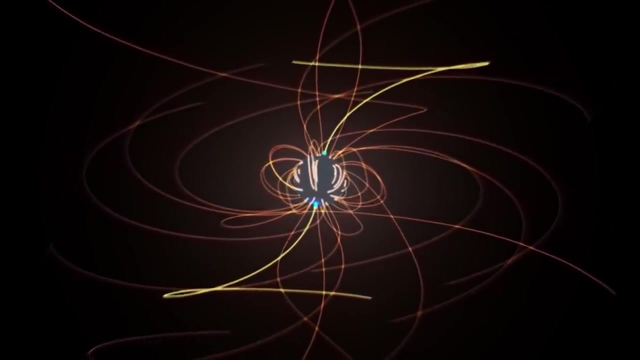 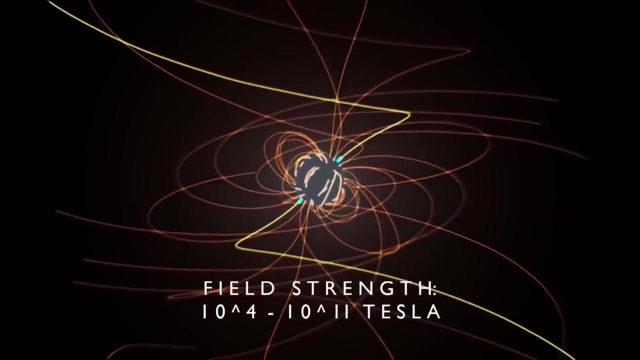 atomic nuclei from decaying, allowing it to remain stable. This internal mass, density and pressure keeps any atmosphere. the neutron star has tightly pressed onto the surface only a few micrometres thick, and this is controlled by the incredible magnetic field produced by the neutron star. The magnetic field of a neutron star can be anywhere between: 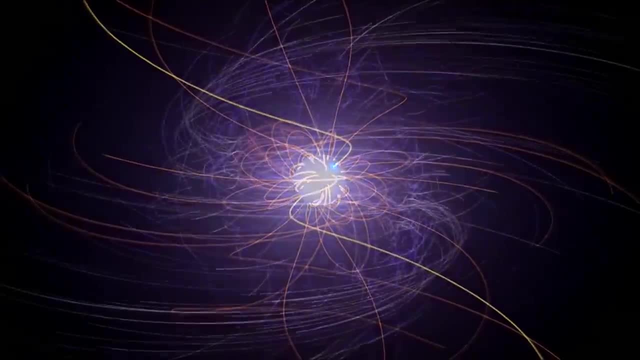 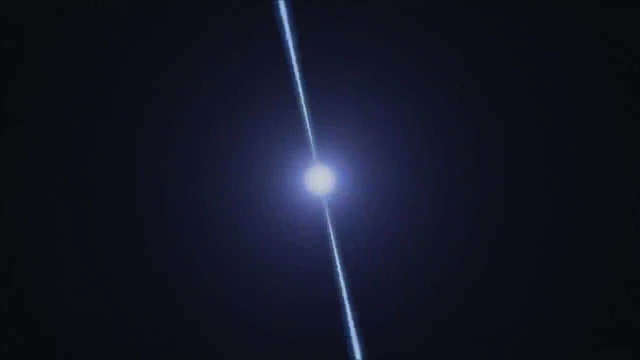 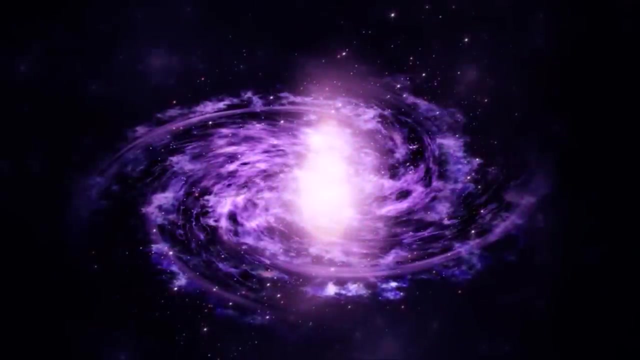 100 million and 1 quadrillion times stronger than the Earth's, making them the most powerful magnetic fields in the known universe has its own terrifying density, mass and attraction, and there could be as many as 100 million of them in our galaxy alone. Most of these are old, cold neutron stars which formed billions. 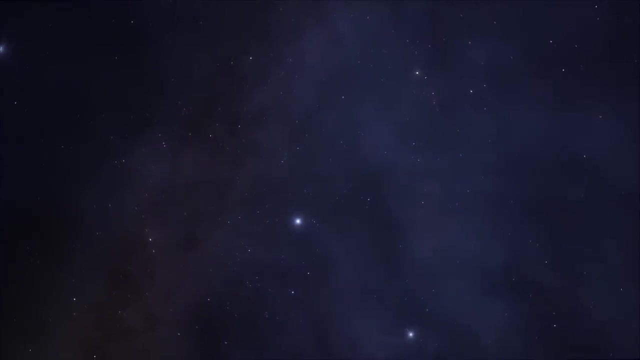 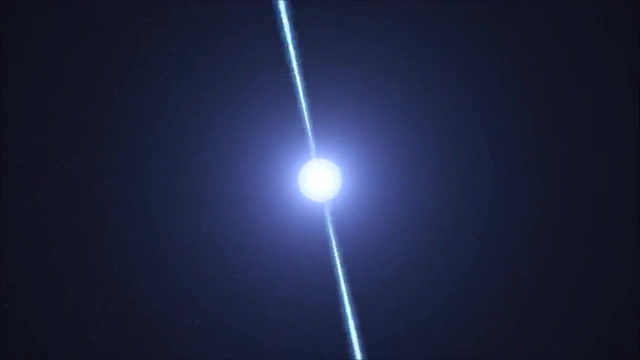 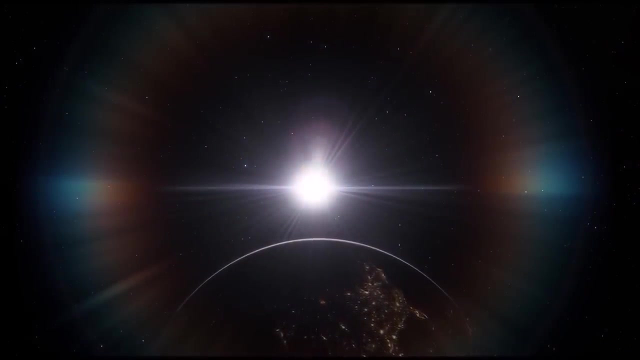 of years ago, but some of them are young and display unique characteristics, especially if they are rotating. All neutron stars emit beams of radiation from their north and south poles, and if those rotating emission points happen to be firing in the direction of the Earth, then we can detect these as pulses of light, Just like relativistic jets firing. 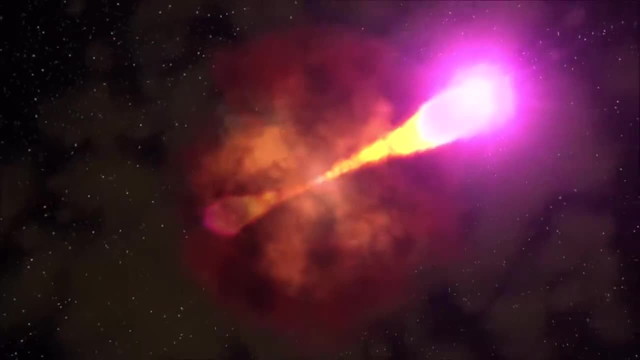 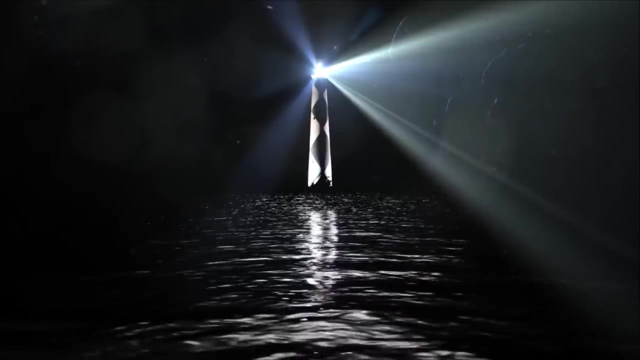 away from crasars. when these beams point in the direction of the Earth, we can detect them from immense distances. When this happens, these neutron stars often resemble lighthouses, firing beams at a consistent rate in the direction of the Earth from all over the galaxy. When 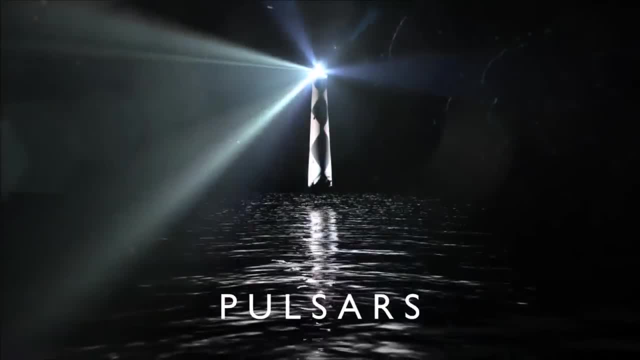 this happens. we call these firing neutron stars, pulsars, and their rotation rates vary depending on their age and what's in their surrounding area. Some can rotate the stars, but some can't, because they're not moving. Some can rotate the stars, but some can't because they're not moving. Some can rotate the stars, but some can't. 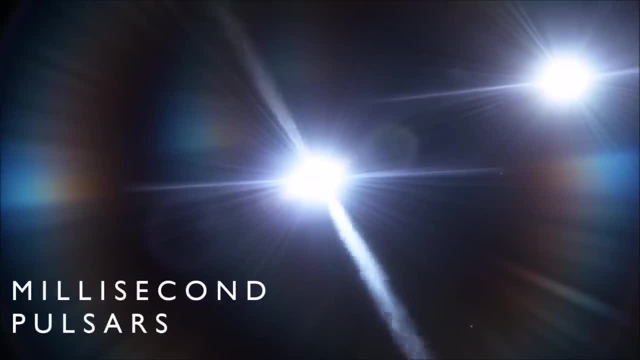 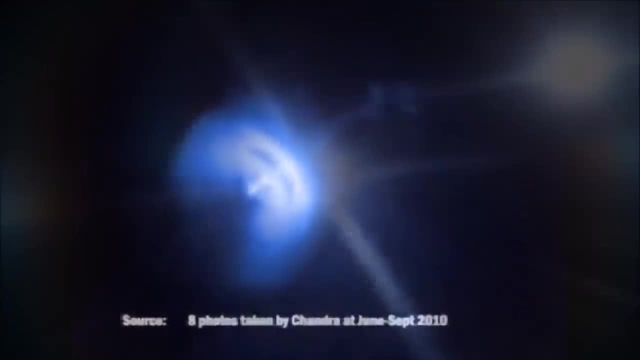 pulsate thousands of times every second and we call the most rapid ones millisecond pulsars, with the fastest reaching speeds of up to 65% the speed of light. The word pulsar literally means pulsating star, and they are named as such because of the pulsing sound they make. 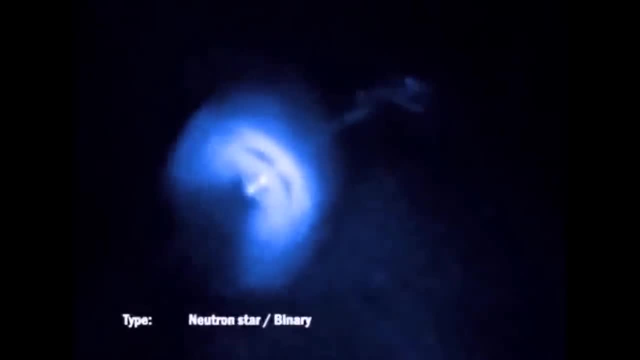 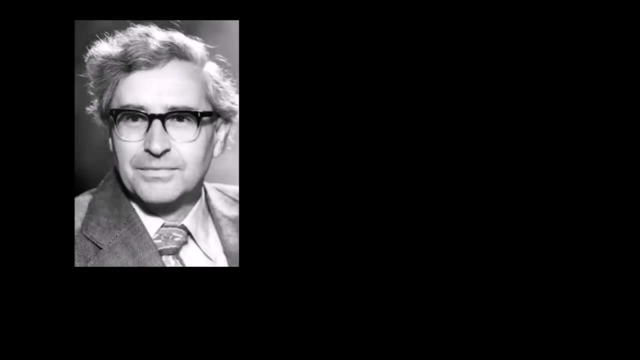 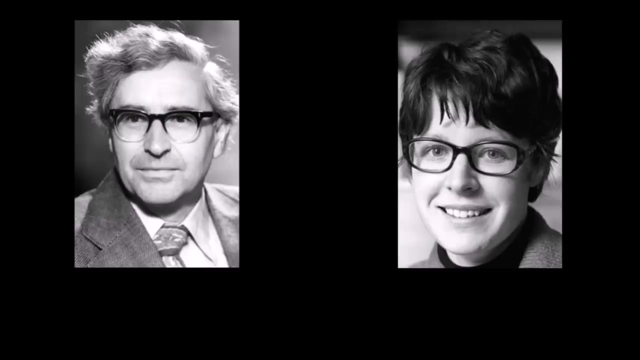 as the beams sweep across the planet in sequence. Following the first noting of neutron stars in 1965 by Anthony Hewish, two years later he and his assistant, Jocelyn Bell Bunnell, detected a radio signal which appeared to be pulsing at a consistent rate, with exquisite precision. In fact, this signal seemed so. 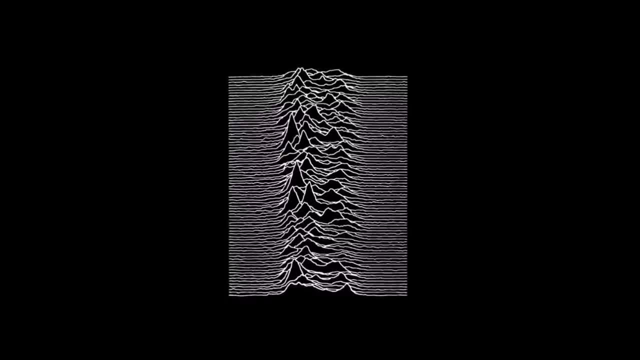 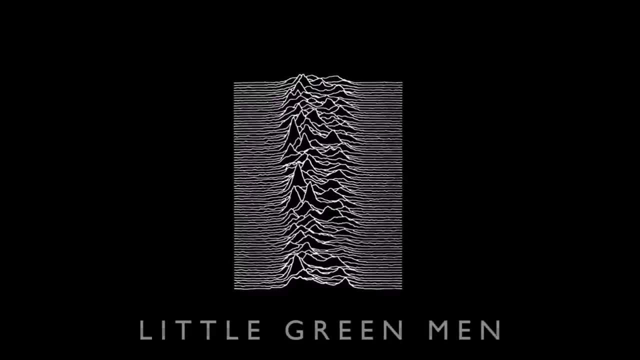 consistent and anomalous that it prompted widespread speculation that Bunnell had intercepted a transmission from an alien civilisation, and so the signal was named LGM1, an acronym of Little Green Men. However, we soon realised that this was in fact a rotating neutron. 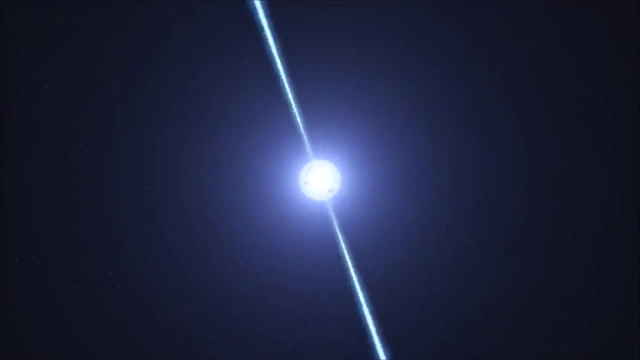 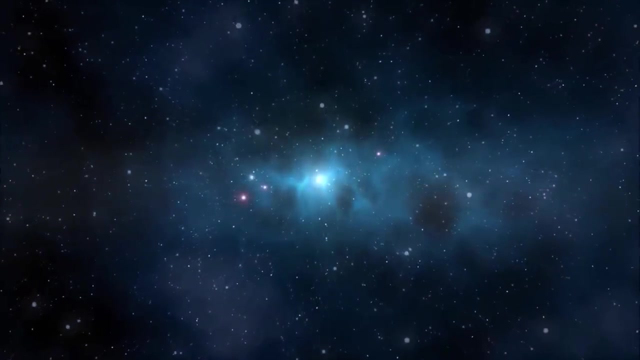 star emitting beams of radiation in the direction of the stars. Since then, we have discovered nearly 2000 of these pulsars, and most are catalogued as part of radio surveys, hence why many of them are named with the prefix PSR for pulsar. 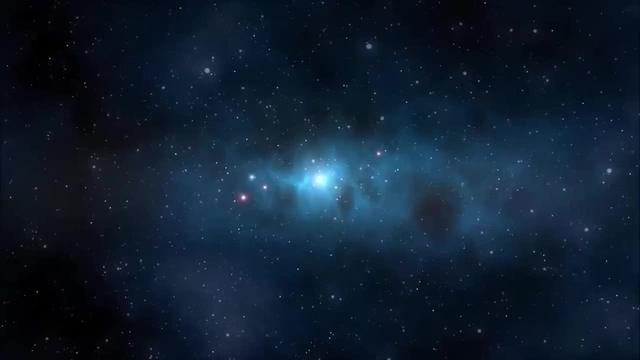 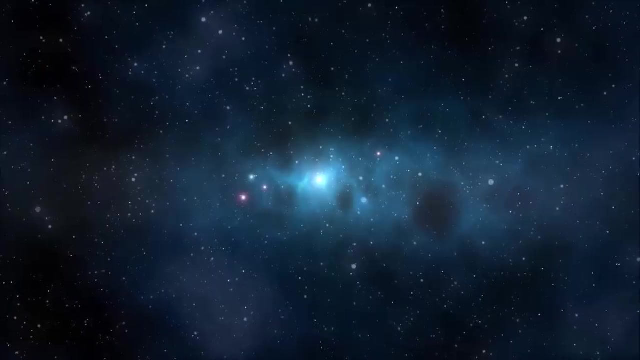 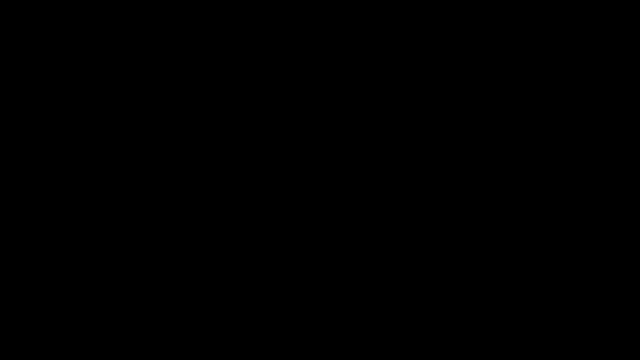 And so LGM1 joined the growing list of astronomical phenomena initially attributed to aliens, but was actually the result of something natural. But fear not, these nuclear lighthouses may yet be of use in the discovery of our species. The Voyager 2 spacecraft is a probe which was launched in 1977 to explore the distant. 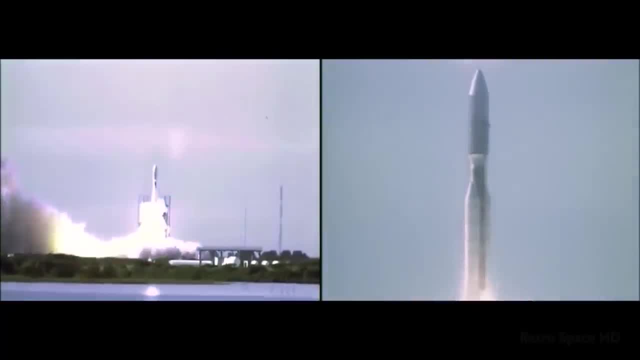 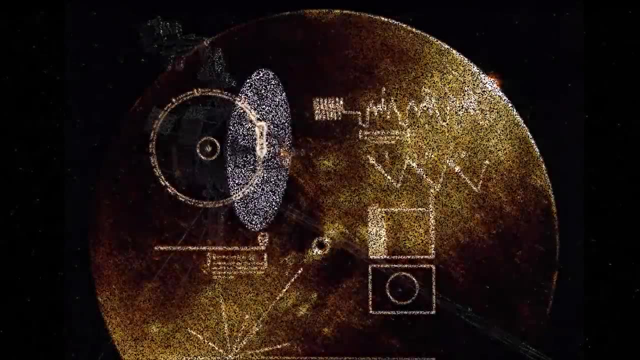 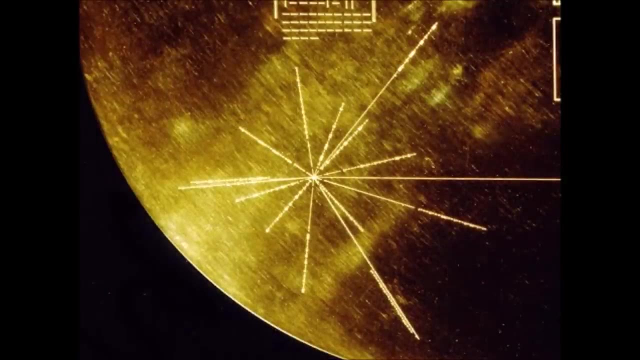 ice giant planets. but since completing this mission, it now barrels through interstellar space, carrying with it a golden record. This record is mankind's CV. It was meant to be found by aliens. It contains information about our location in the galaxy. This map was created. 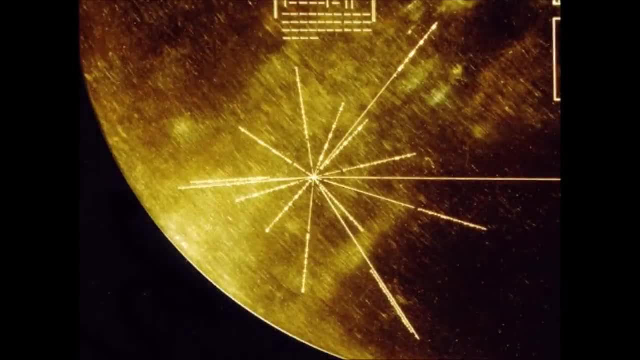 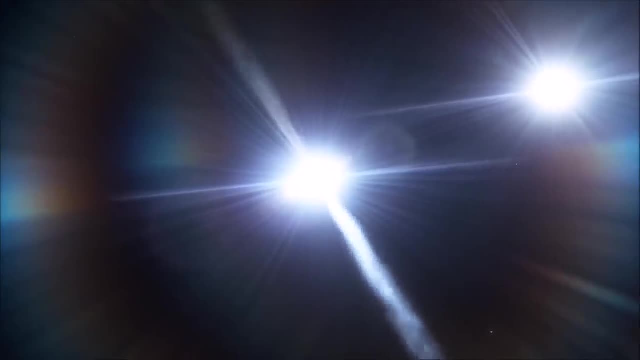 using pulsars as a point of reference, because they are extremely good timekeepers. While their positions may change, they are still very important to us. While they are extremely important to us, their pulse frequency remains highly consistent. So the idea is that a civilization 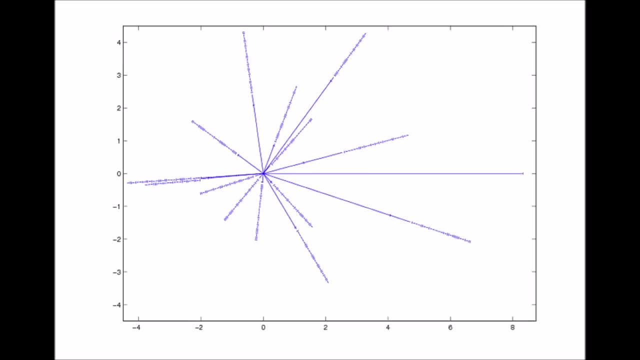 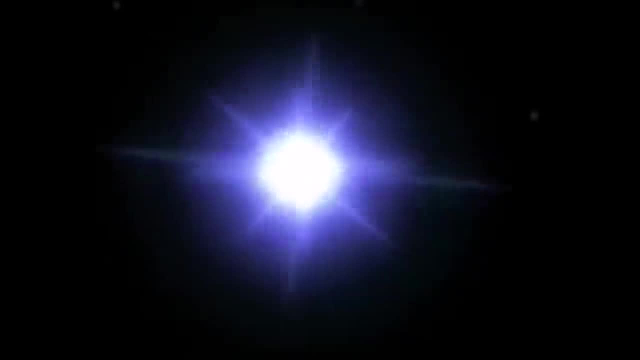 could look at this map, which shows the position of Earth relative to 14 nearby pulsars, and they could find these pulsars based on their pulsation rates, which we have attempted to inscribe on the record, and then reverse engineer our position. It's a genius idea, or at. 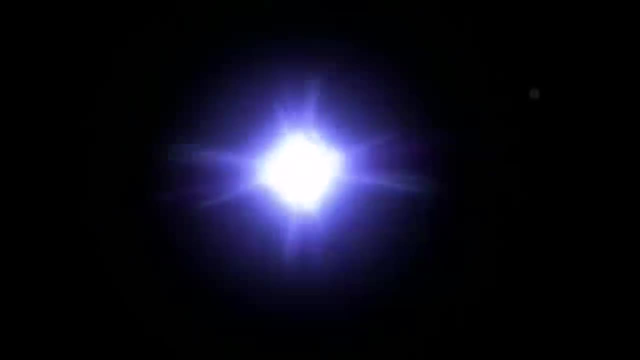 least, it seemed that way in 1977. But in the years since, we have learned that there could be hundreds of millions of these pulsars in the galaxy, and though their rates are relatively consistent and measurable, they are still very important to us. 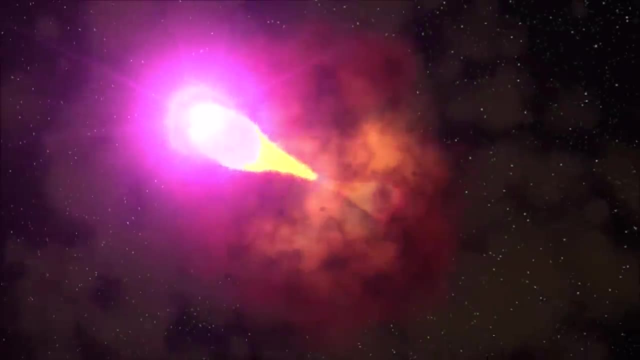 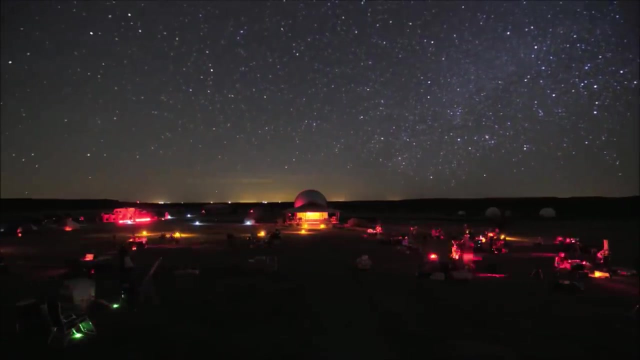 For example, the direction in which they fire can change unpredictably, meaning a bright beacon which once illuminated the Earth with flashes of radio energy may just become another silent speck in the night sky. Finding 14 coincidentally placed pulsars in a galaxy. 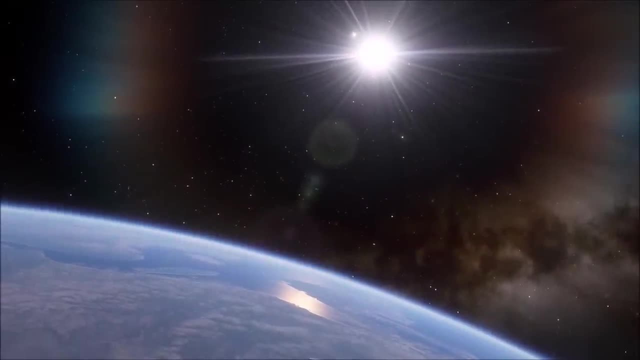 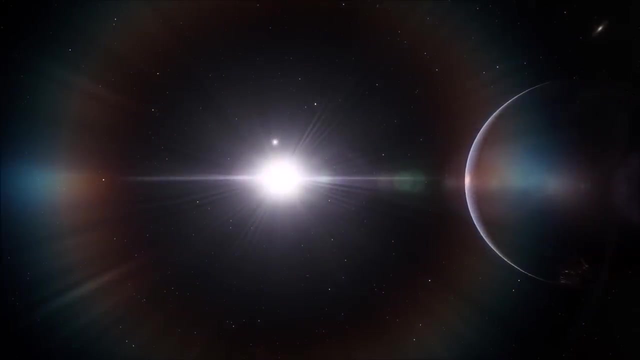 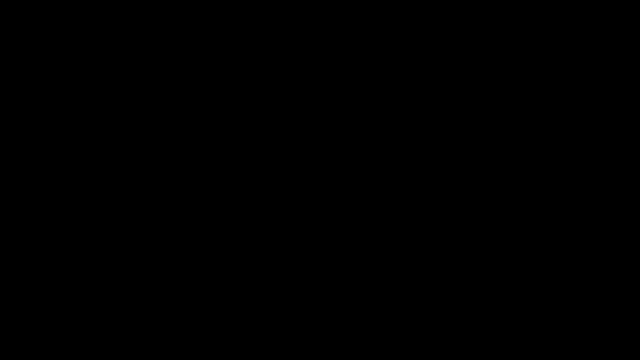 with potentially billions, isn't even comparable to the needle and haystack analogy. So whatever and whoever Voyager might encounter on its journey, they'll likely never be able to work out where the probe came from, even if they manage to decipher the map. The faster a neutron star rotates, the stronger the magnetic field it generates, and for 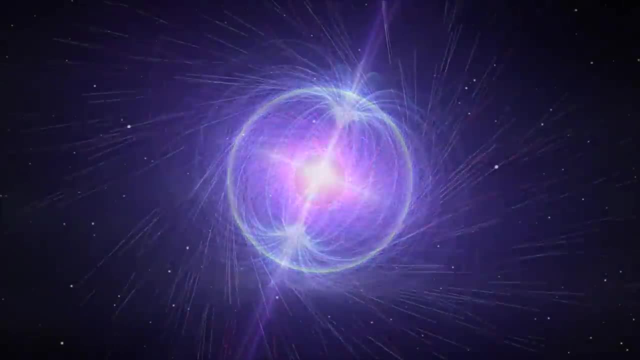 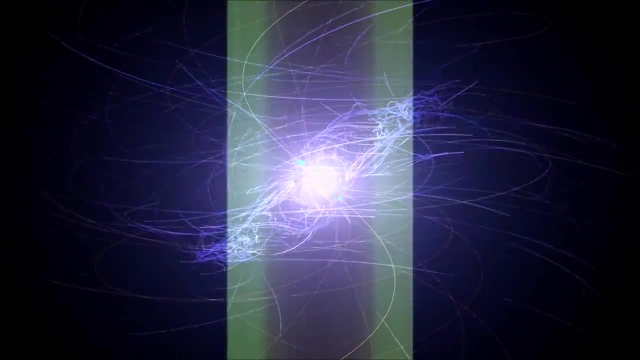 those exceptionally extreme neutron stars. there is another classification: A magnetar. These are similar in size and mass to neutron stars, but rotate so fast that they are even more extreme and deadly. Magnetars can be caused by the supernova that created it or 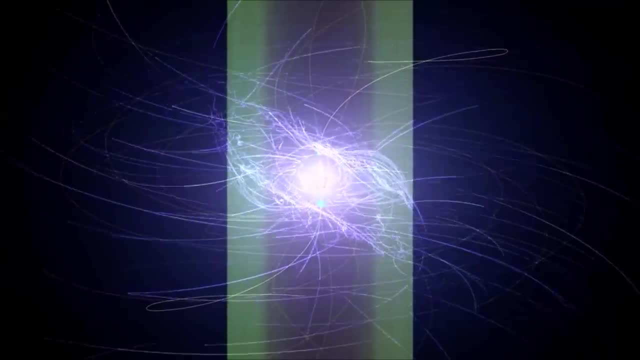 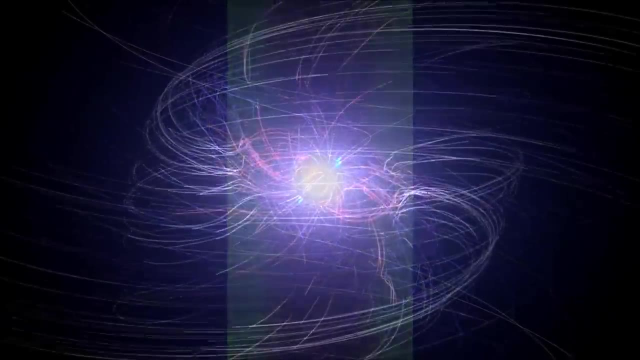 by the gravity of a neighbour around the neutron star. Whatever the case, their magnetic fields are modified, exceeding 1,000 times the strength of a normal neutron star's field, which is already billions of times the strength of the Earth's. It's a scale difficult to. 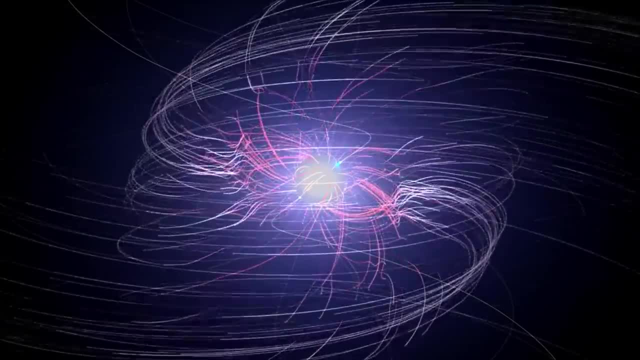 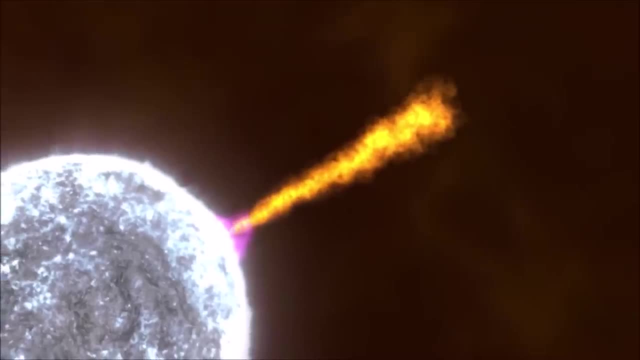 fully appreciate. These fields are so intense that they often experience very strong x-ray bursts, and when their shells crack, blasts of x-ray and gamma radiation are emitted. This can cause an aptly named starquake, which can lead to a storm of solar energy trillions. 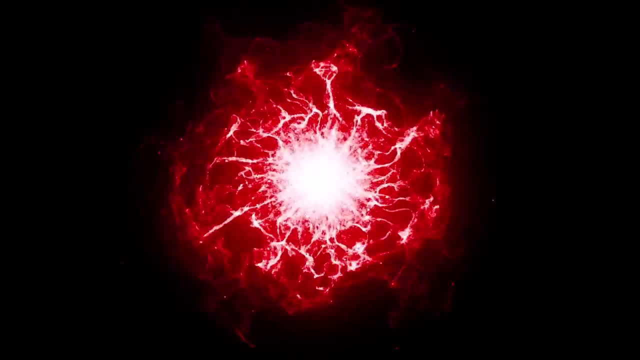 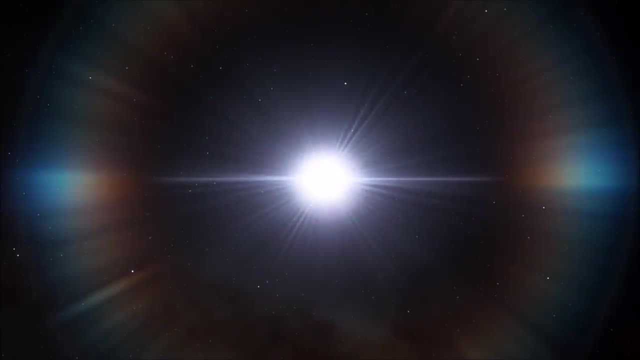 of times more powerful than the solar emissions of our own star. Unsurprisingly, these magnetars are not very stable. The strong magnetic fields tend to break down after about 10,000 years, which is only the blink of an eye on a cosmological timescale, and it is a much narrower window. 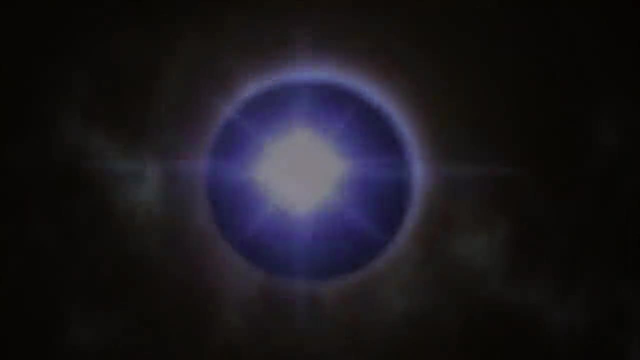 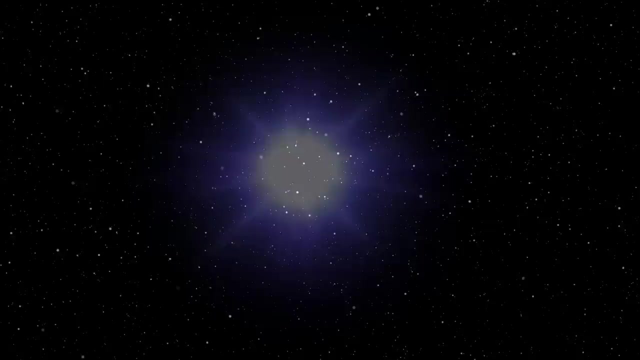 for us to exist, to observe them. Therefore, magnetars are considerably rarer than neutron stars and pulsars. There are estimated to be about 30 million inactive magnetars, based on the number we can currently observe. Most neutron stars are old, spinning much more. 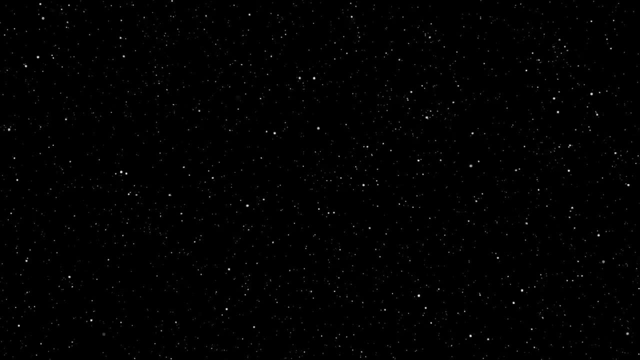 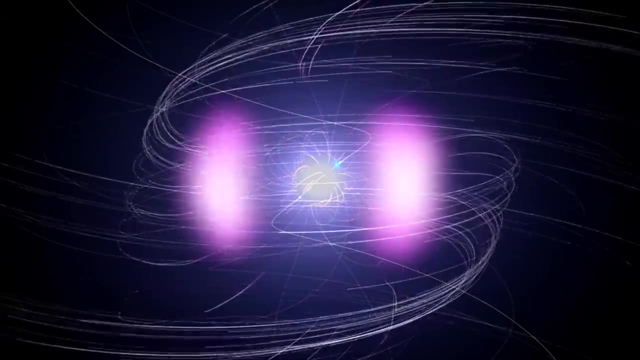 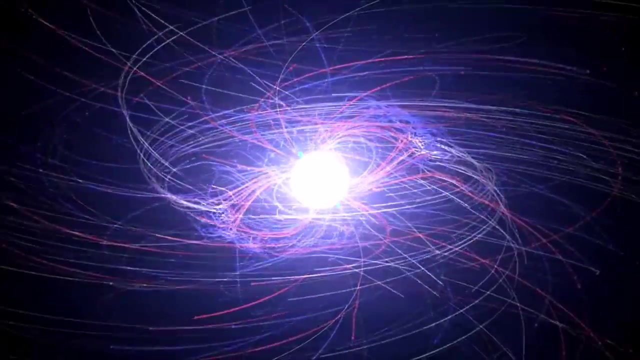 slowly than the young magnetars and millisecond pulsars. So the question is: what is the difference between a neutron star and a pulsar? Well, the answer can be all three. Loads of weird and wonderful things can happen to a neutron star, especially if we give it a neighbour. 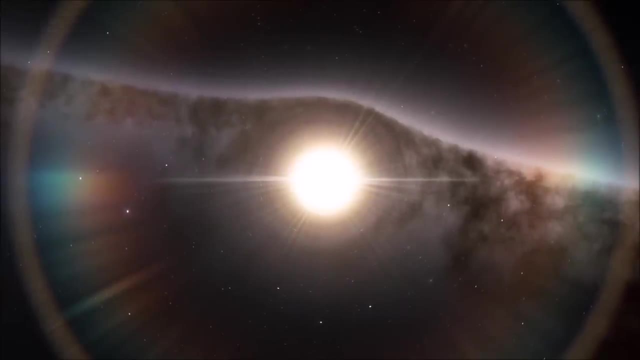 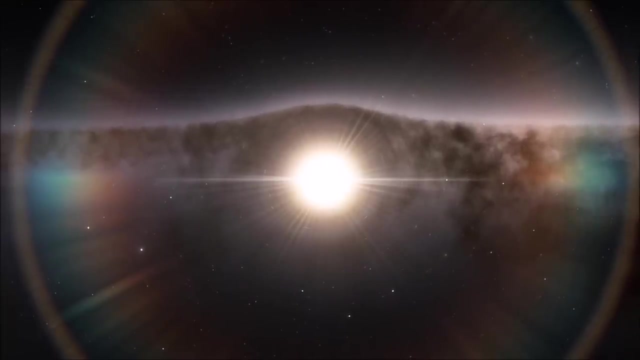 Neutron stars can continue to gain mass and grow after formation, and they grow in the same way that planets and moons do, through accretion- the gradual accumulation of matter as the object orbits. Neutron stars have an insanely strong gravitational influence and therefore attract a lot of extra mass from their surrounding. 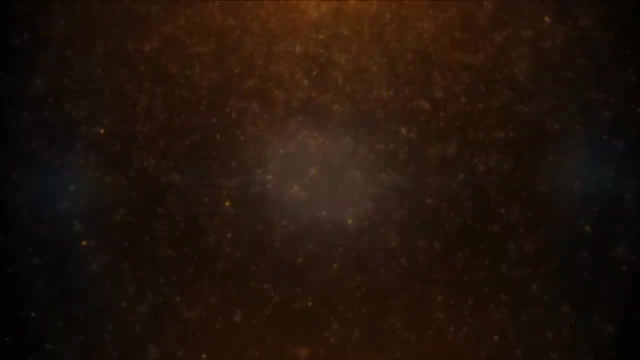 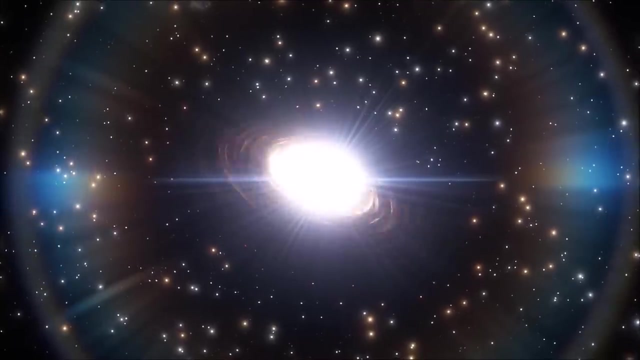 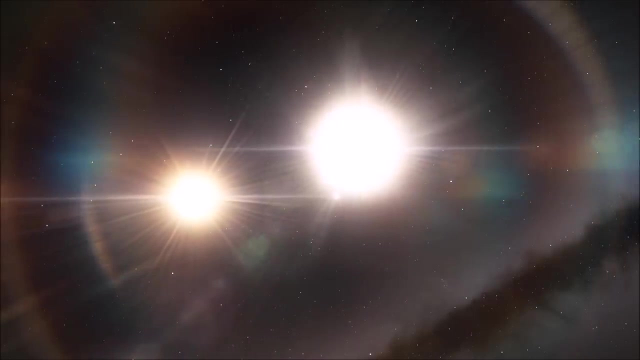 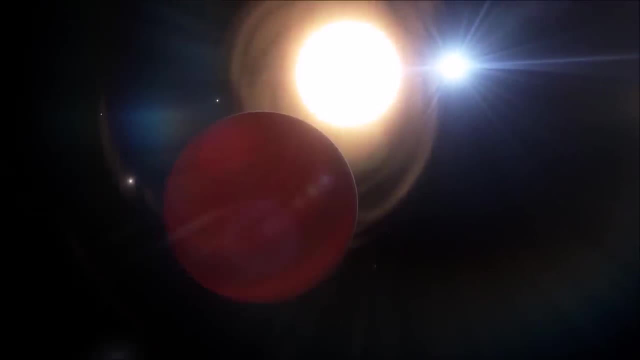 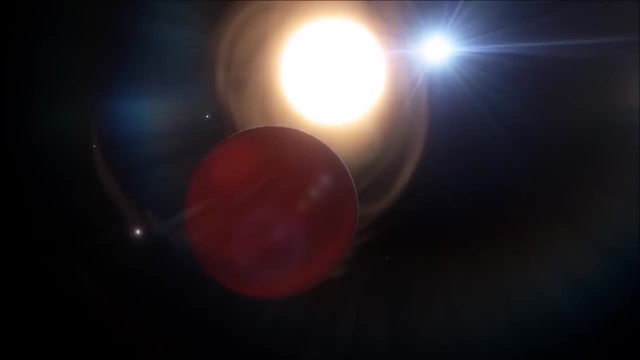 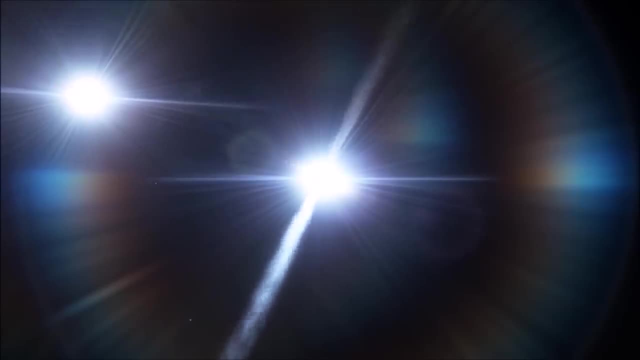 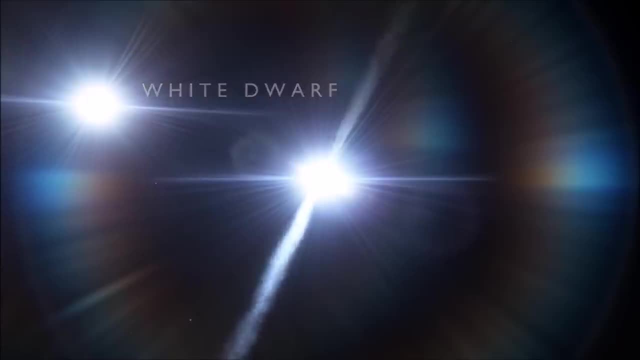 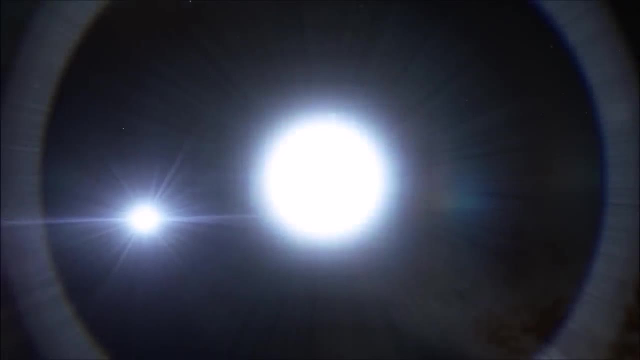 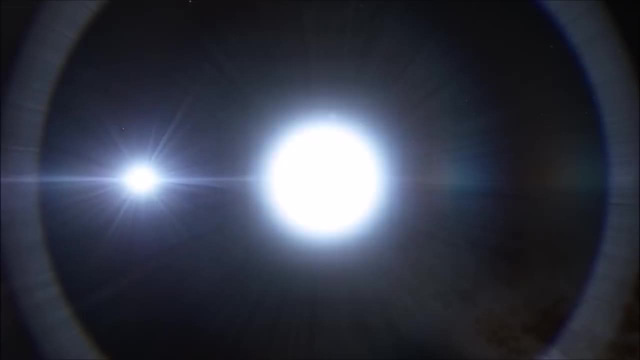 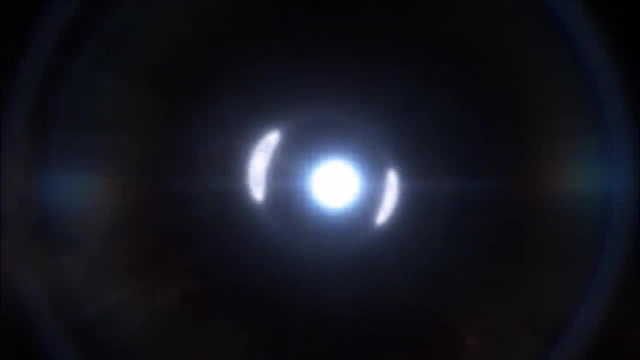 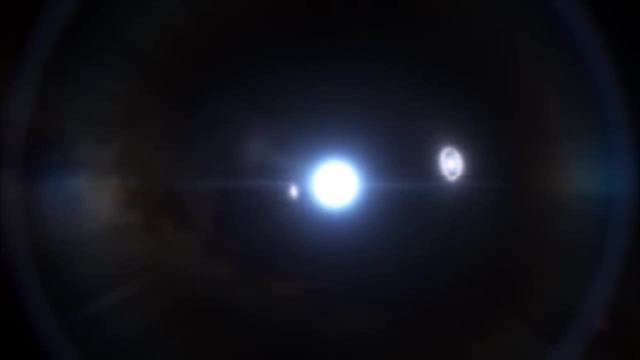 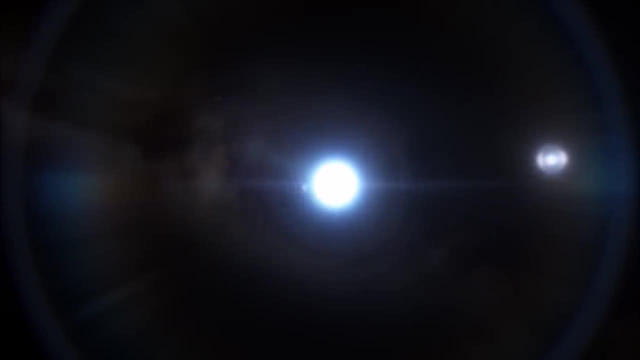 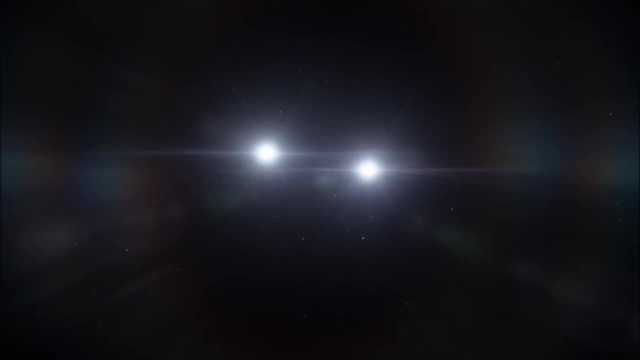 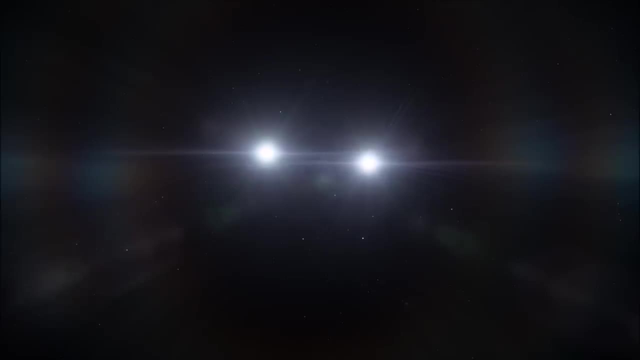 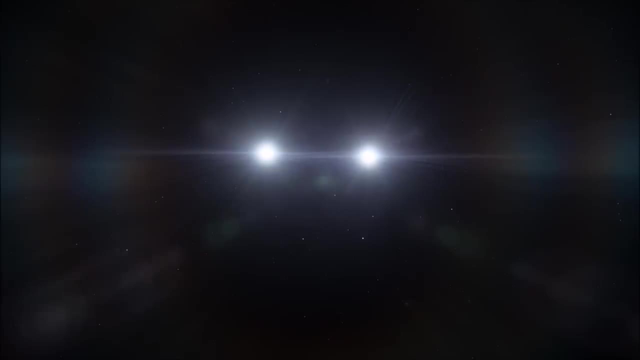 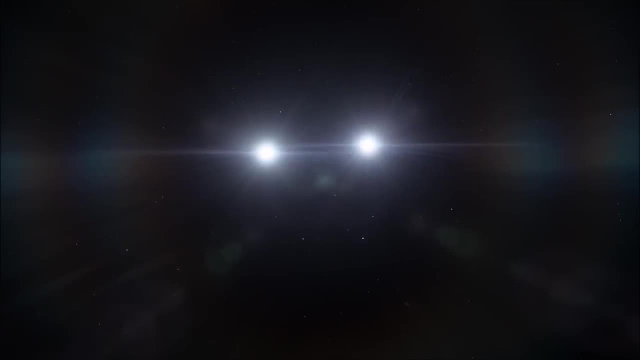 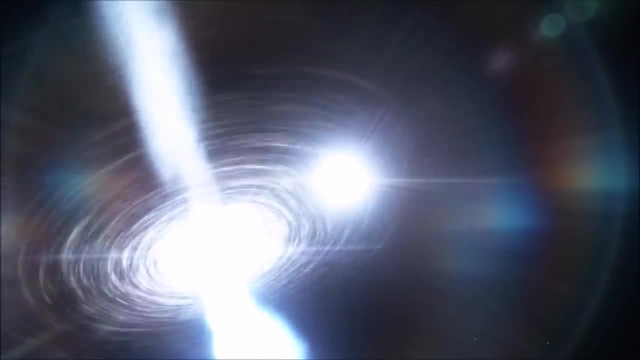 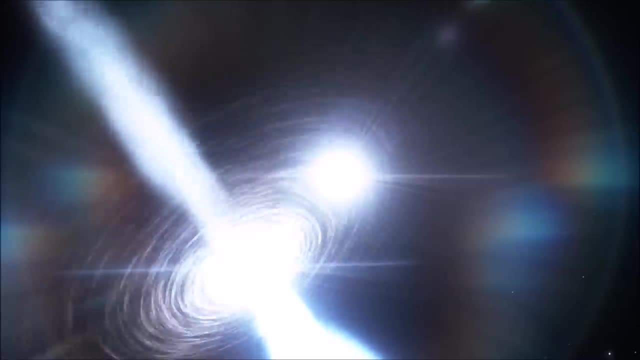 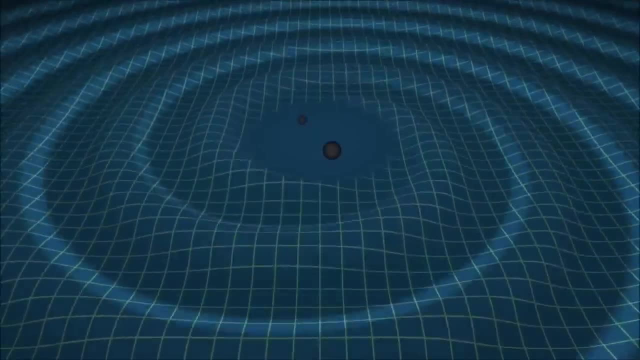 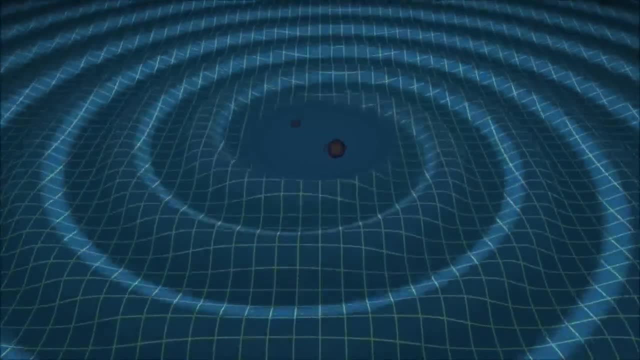 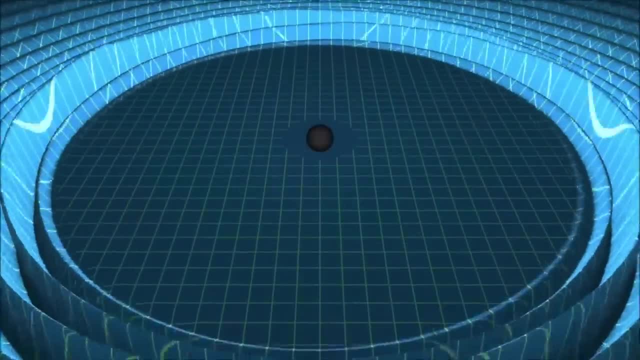 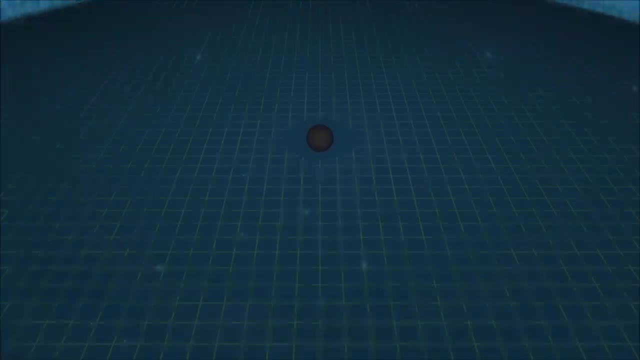 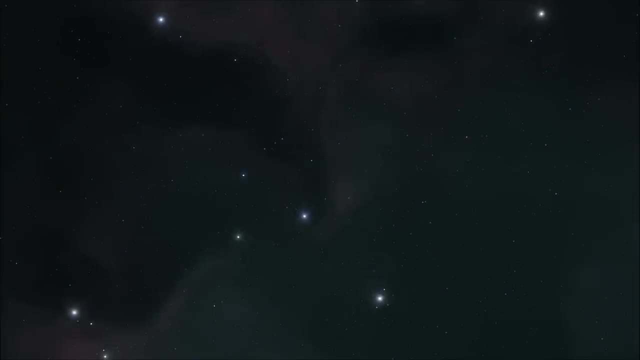 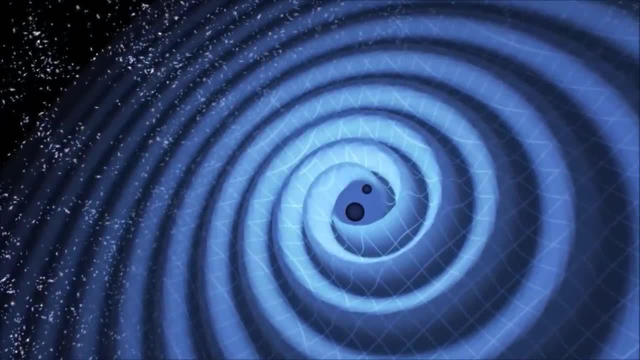 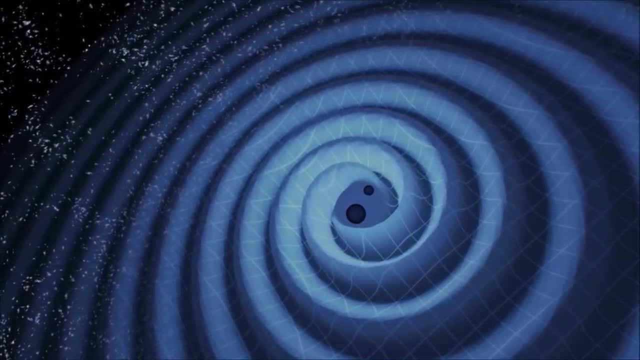 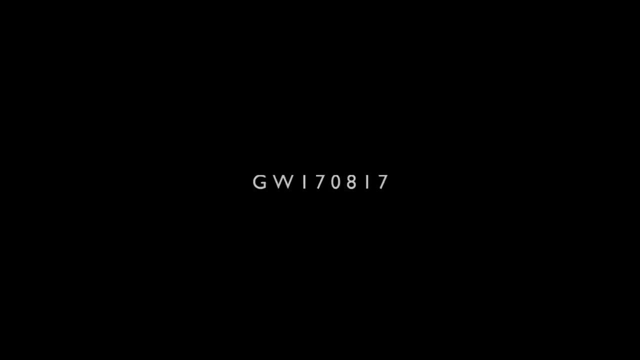 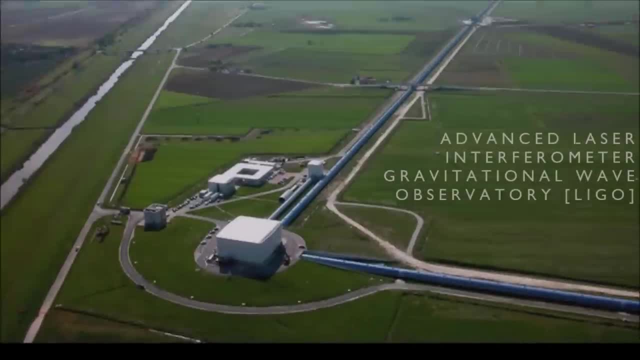 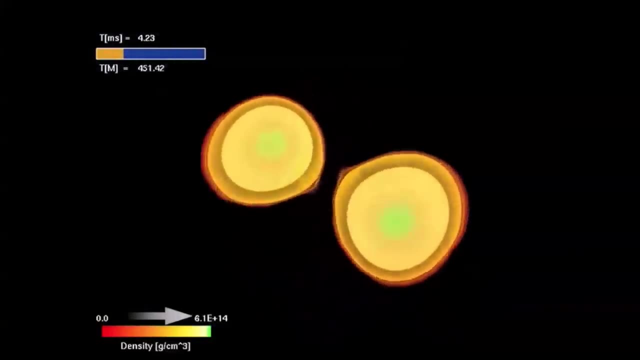 name of a gravitational wave signal which was detected by the Advanced Laser Interferometer Gravitational Wave Observatory, or LIGO, and scientists believe that these ripples in space time are the result of two neutron stars colliding in a galaxy over 140 million light years away. 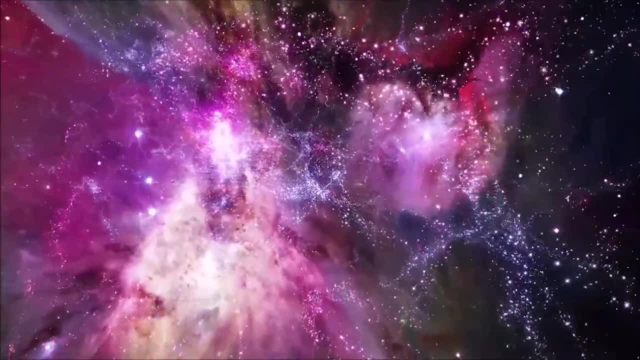 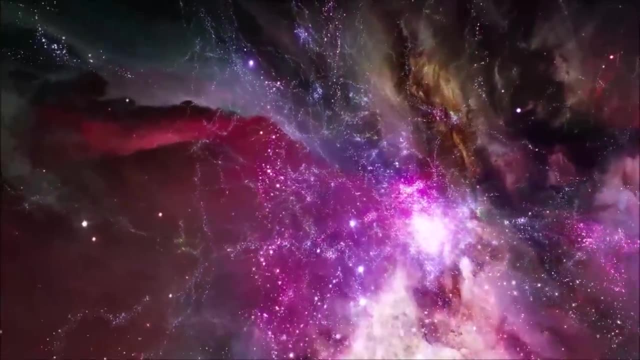 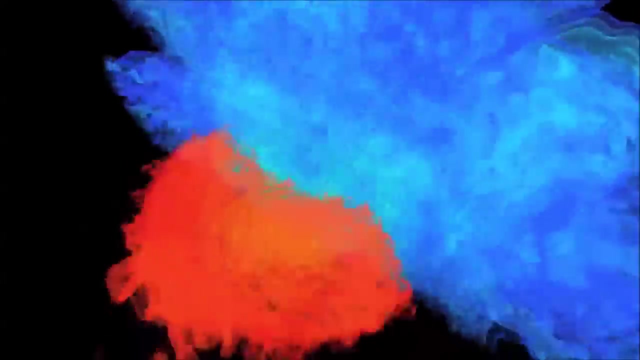 With detectability across such vast distances, it should come as no surprise that the actual collision is just as terrifying and far-reaching. When the two neutron stars are within touching distance, the tidal gravitational forces of each shatter the outer shells, releasing the enormous reserves of matter trapped within into space, which is under considerably less. 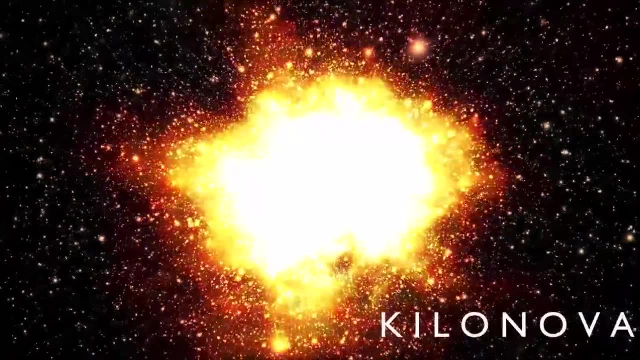 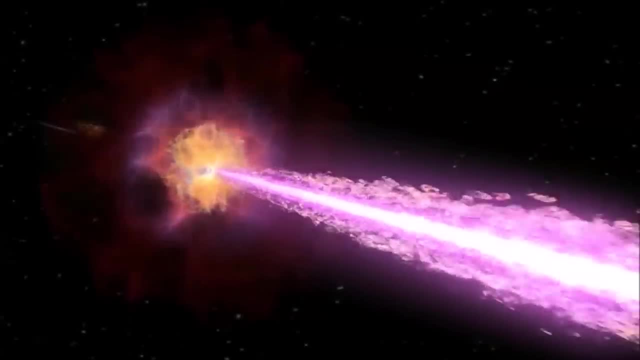 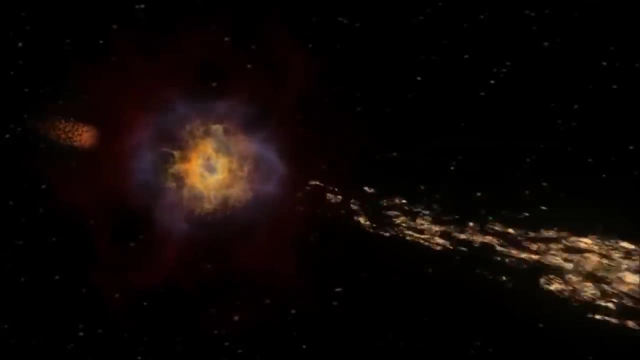 pressure and explodes in an appropriately named kilonova explosion. This explosion is a source of short gamma-ray bursts, the most destructive electromagnetic explosions in the universe. After this cataclysmic explosion has taken place, the two merging neutron stars will do one of two things: They will either become a more massive neutron star or the 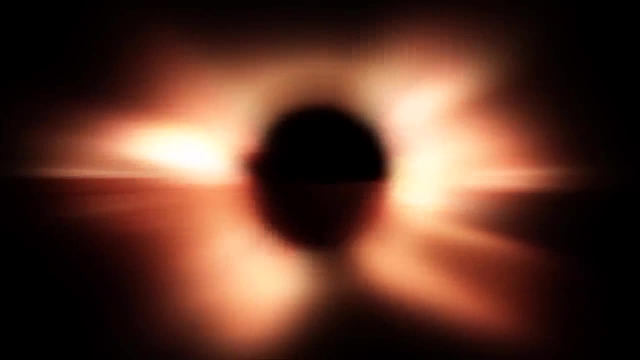 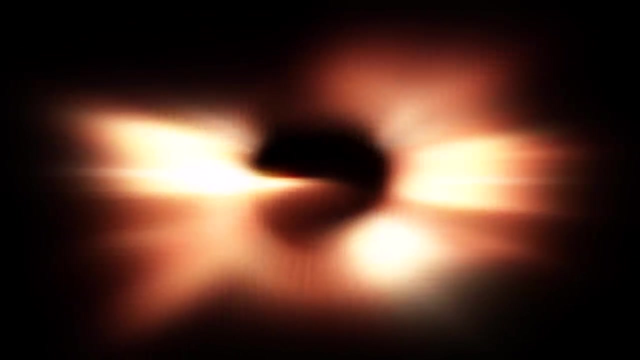 two masses will merge into one, The two stars will collapse and form a black hole. The lower bound mass limit required to form a black hole is between four or five times the mass of our sun. If the two neutron star cores combine but remain below this mass, then they will combine to form a magnetar. 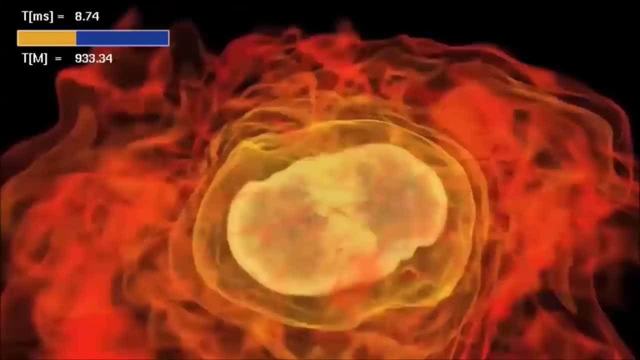 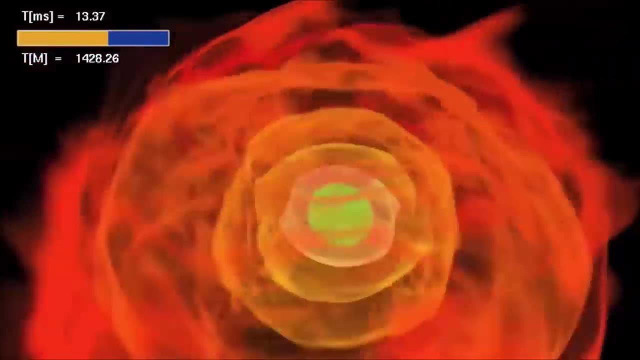 with a magnetic field trillions of times stronger than the Earth's. Alternatively, the two dead stars will collapse in on each other and form a black hole which is infinitely dense at its singularity. It's an intriguing and bewildering process, but the merger of neutron stars is actually. 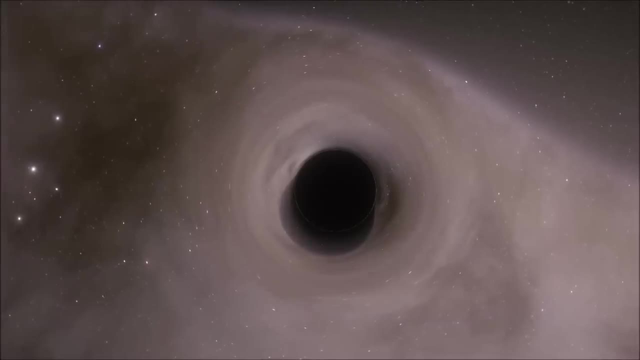 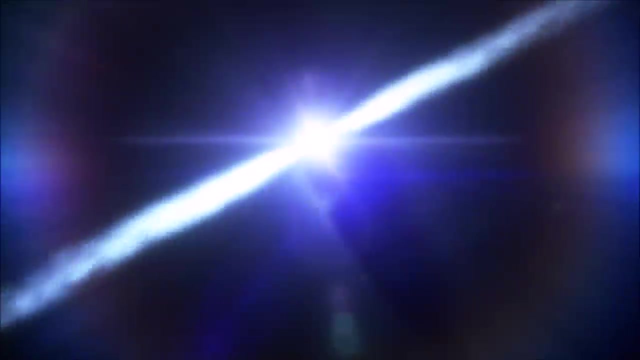 quite a fruitful event. The shattering of neutron star shells releases loads of heavier elements, which were fused by the star that came before it, and these heavier elements mix into the clouds of hydrogen and helium gas in space, the same clouds that form planetary systems, The remains of kilonova. 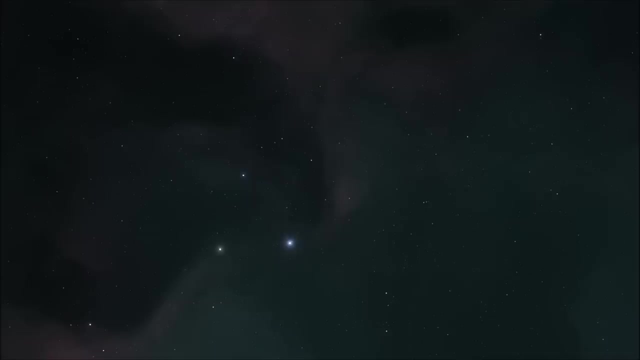 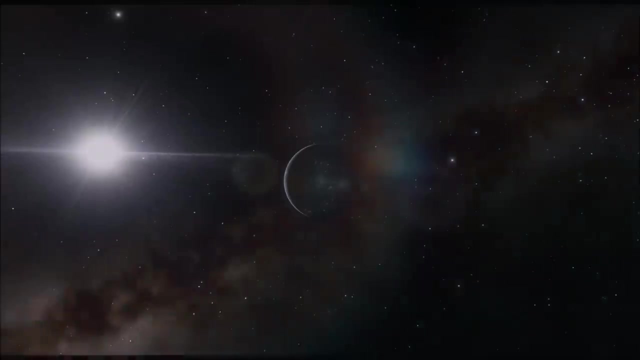 explosions is likely the source of most of the heavy elements in the universe, and the solar nebula cloud, which our solar system formed from five billion years ago, likely contains the remains of neutron stars which exploded billions of years before in a profoundly younger universe. Neutron stars are just another tiny, improbable piece of the unendingly 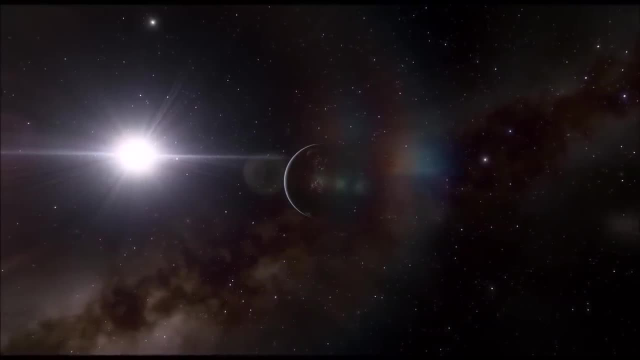 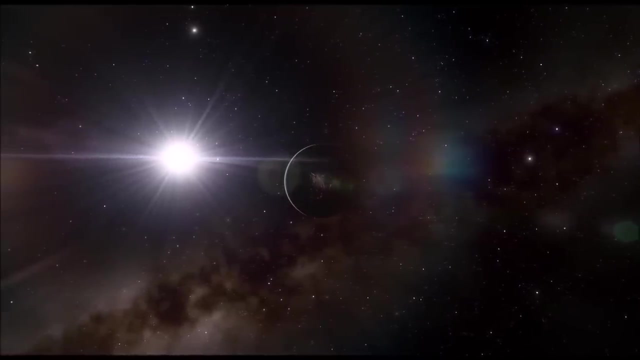 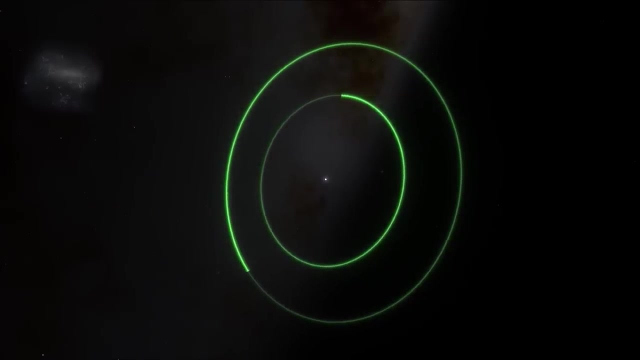 complex puzzle that is the emergence of life from stardust. Speaking of planetary systems, what would it be like for a planetary system orbiting a neutron star? We've observed planets around neutron stars before We detect them when said planet passes in front of the beams of a firing pulsar. As such, we refer to them. 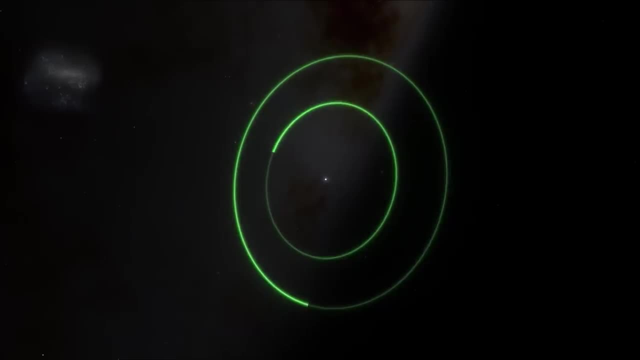 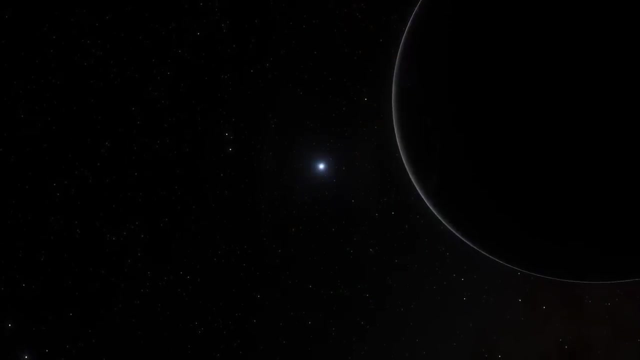 as pulsar planets, and we've known about them since 1991 and have discovered entire planetary systems orbiting them since then. It's unlikely that these were the planets that orbited the star in the main stage of its life. On the contrary, all of the pulsar planets we have observed fall into three main 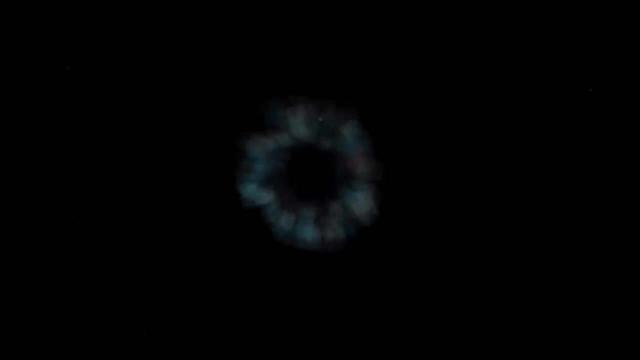 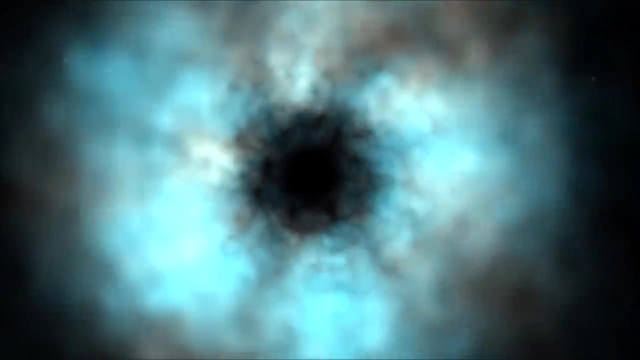 groups, the first being planets which formed out of the metal-rich debris left over from the supernova explosion, which formed the neutron star. Or the planet could be a captured planet. The extreme gravity of a neutron star may just be enough to pluck a hurtling rogue planet. 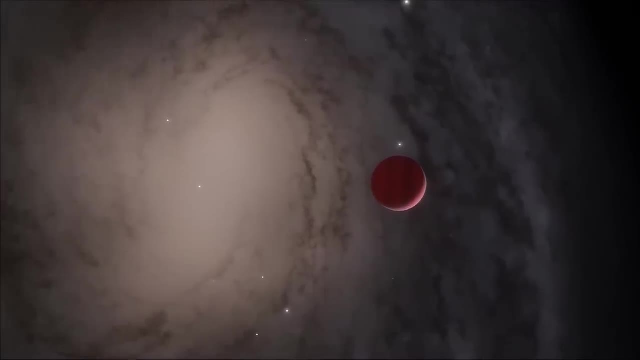 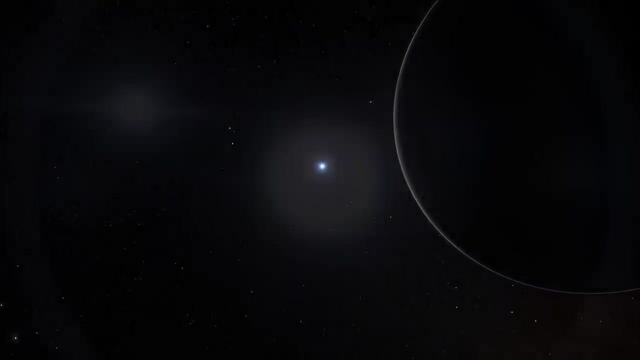 out of the darkness of interstellar space and into orbit, damning it to be radiated, ravaged by its new deceased host, 3.. The planet might actually be the other star in the binary system which used to orbit the pulsar, but that has been stripped down. 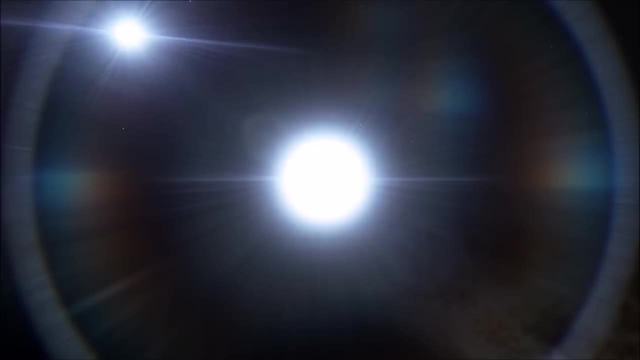 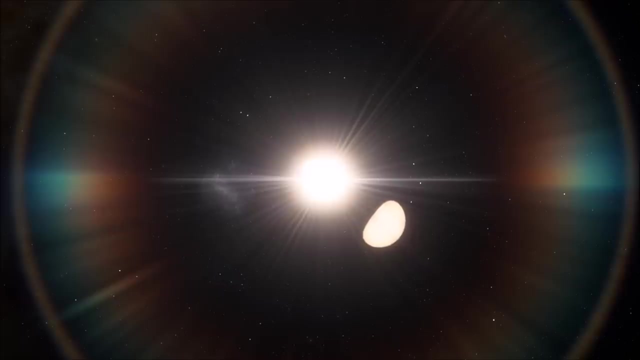 and solidified due to the extreme irradiation of the pulsar. In 2011,, we discovered the companion of the pulsar, PSR J1719.. It was a white dwarf star in the final stage of its life, but it had most of its mass torn off by the pulsar it. 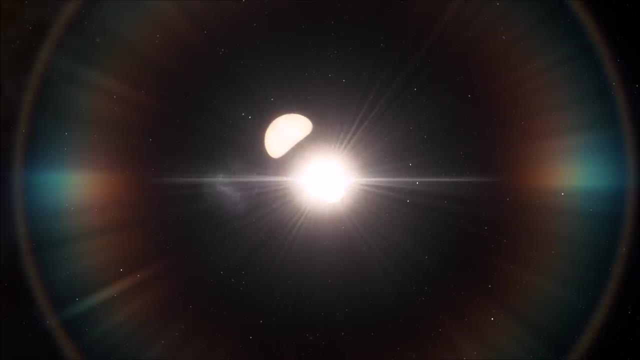 visits and was spiralling inwards towards its companion, destined to be shredded up and ripped to pieces. However, this star orbits its neighbour in an unlikely position, at a distance slightly smaller than the radius of the Sun, just under 700,000 kilometres. 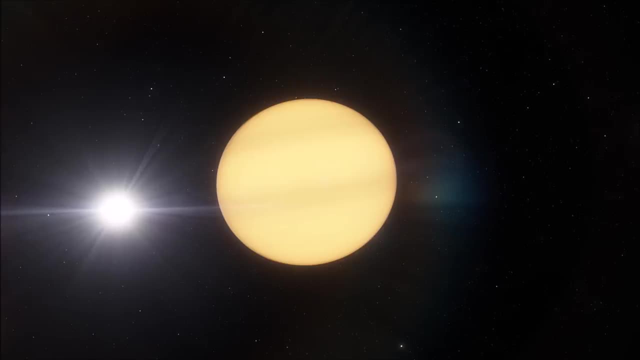 This isn't close enough to shred the planet entirely, but the pulsar's influence is so strong that the carbon in the star has likely crystallised. The neutron neighbour is now likely a diamond planet five times the size of the Earth. 3. The pulsar is a star in the binary system, but it's not a star in the binary system. The pulsar is a star in the binary system, but it's not a star in the binary system. Life on these neutron star planets is non-existent and hopeless. Those planets lucky enough to escape total destruction are subjected to torturous conditions: The beams of gamma. 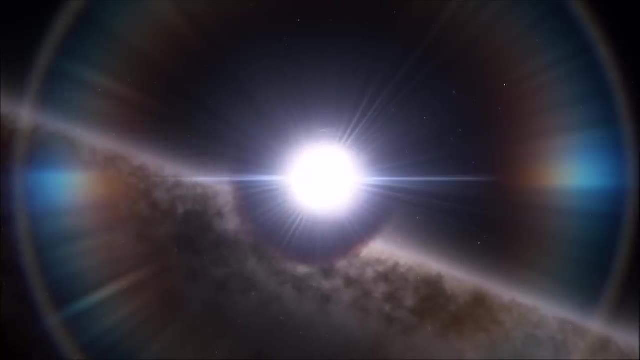 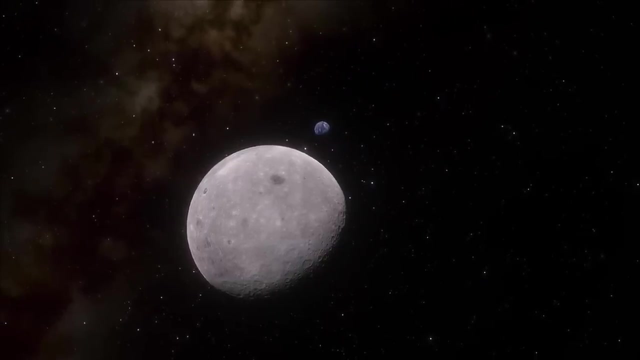 radiation, X-rays and extreme solar energy would ravage any planet. If a magnetar came within range of our planet, say about the distance of the Moon, then you would start to notice fast. Our atoms would be warped and would change shape, completely destroying. 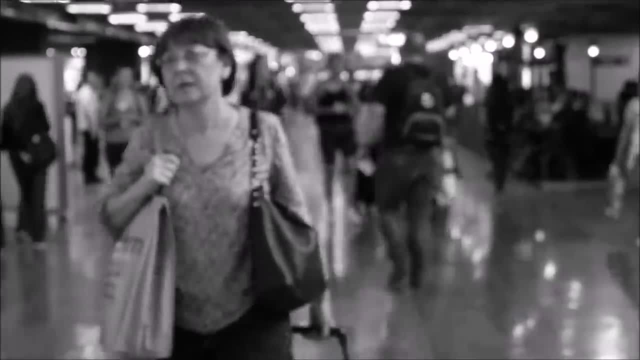 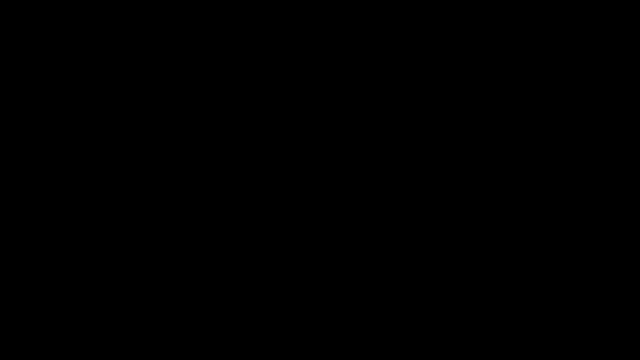 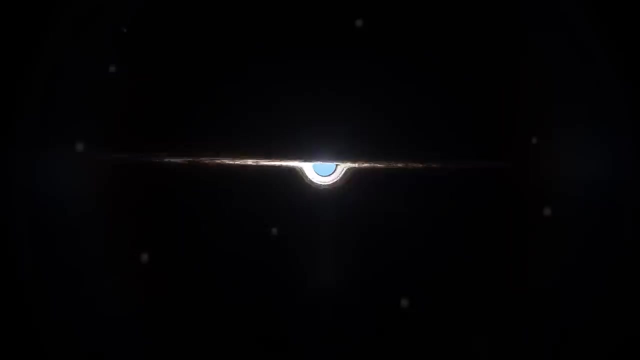 your molecular structure and dissolving your body. Nothing can survive under the vice like grip of a pulsar or worse, a magnetar, And so the final question is: if neutron stars are virtually unbreakable and composed of the hardest materials in the universe, then what happens when the immovable object 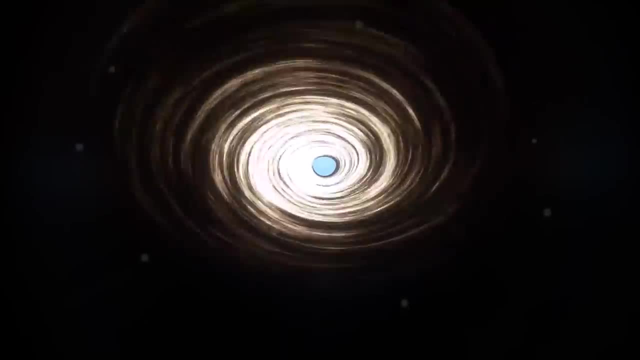 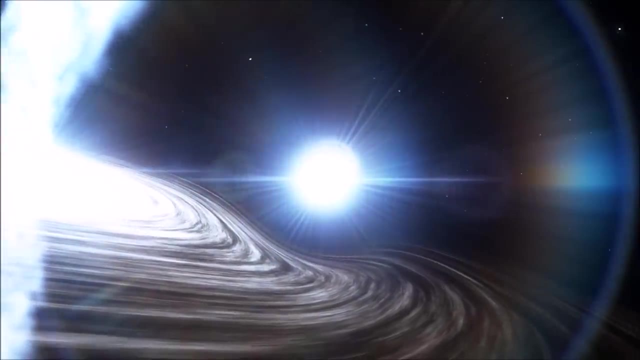 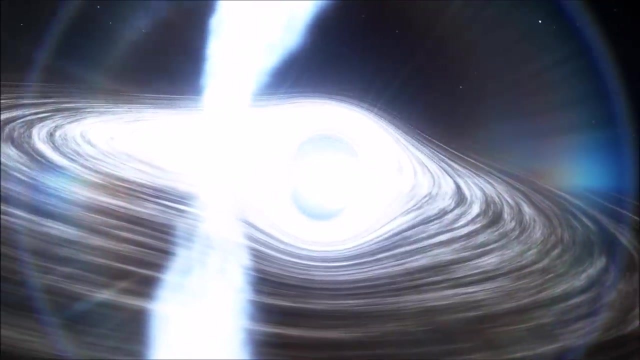 meets its unstoppable force. What happens when a neutron star is consumed by the only thing stronger and more powerful than itself- a black hole? Well, we may finally have an answer. Only a few months ago did those stars appear in those same gravitational wave observatories in Italy pick up more ripples in space-time. 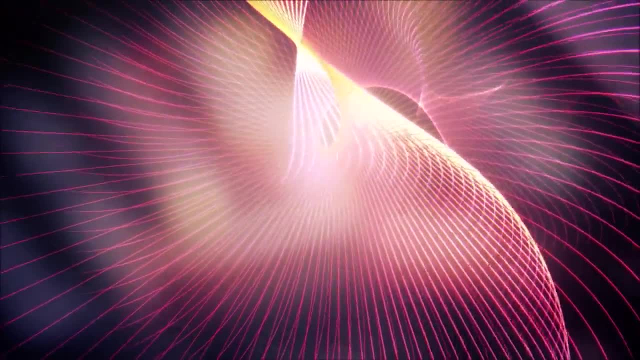 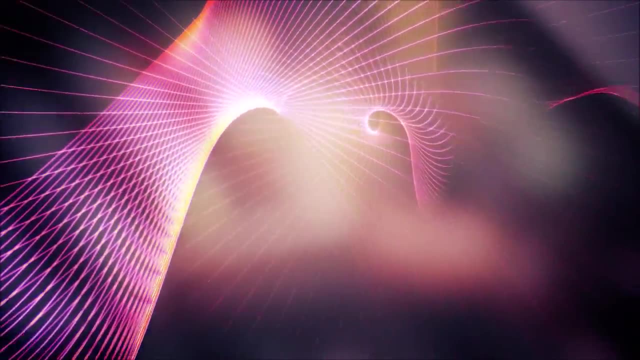 More gravitational waves created by a collision a little under a billion light years away. The signal is named S190814-BV and is believed to be the product of a neutron star being eaten by a black hole. Scientists analysed the wave patterns from the two objects and 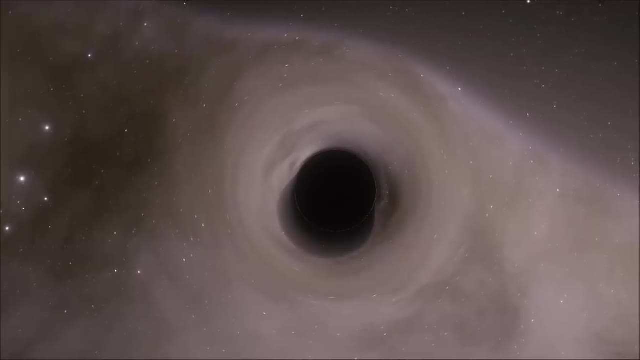 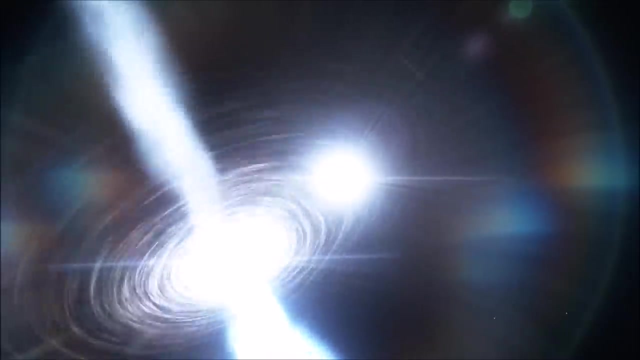 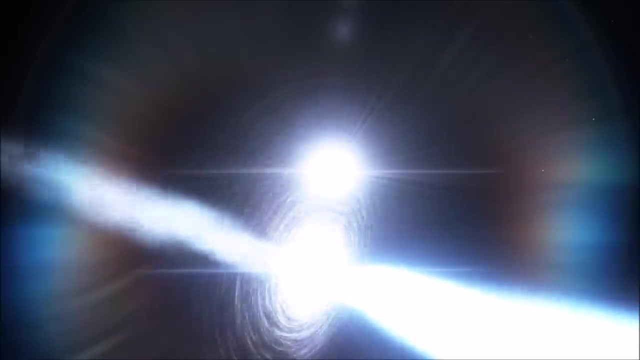 determined that one of the objects must have exceeded 5 solar masses, while the other was some way less, Likely meaning that this is a black hole and neutron star. Regardless, the waves were a product of the moments before the collision. As for the 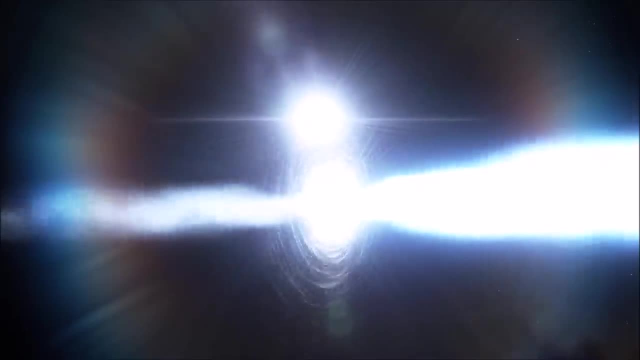 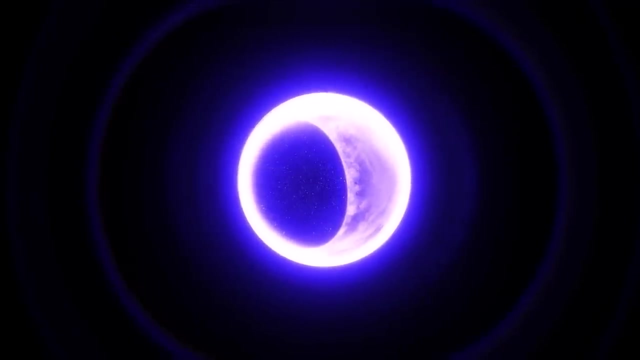 collision itself. Well, if the black hole in question is large enough, then the neutron star could disappear over the event horizon with one big gulp. This would release no energy beyond the boundary and would be somewhat anticlimactic if you were an observer looking. 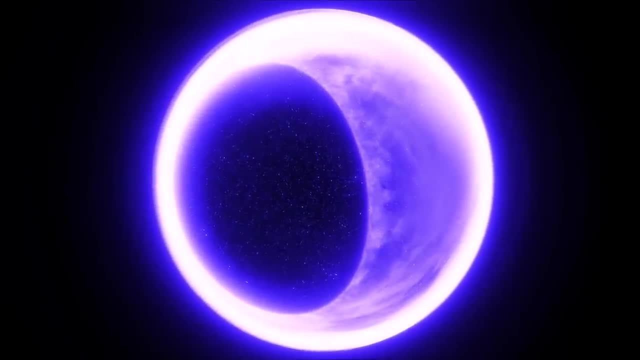 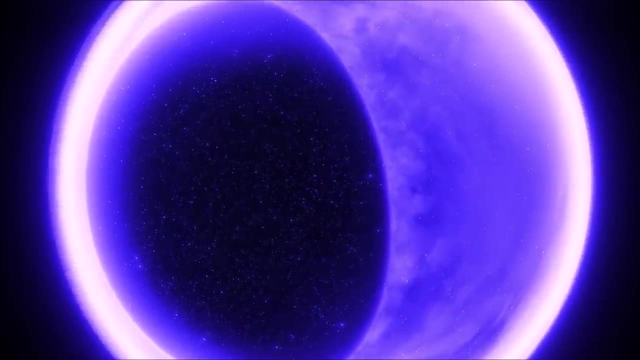 on from the outside. In this case, however, it's unlikely that the mass difference between the two is sufficient for the black hole to be capable of such a large gulp. so some impact would have occurred: The neutron star would be ripped apart by gravity and its matter. 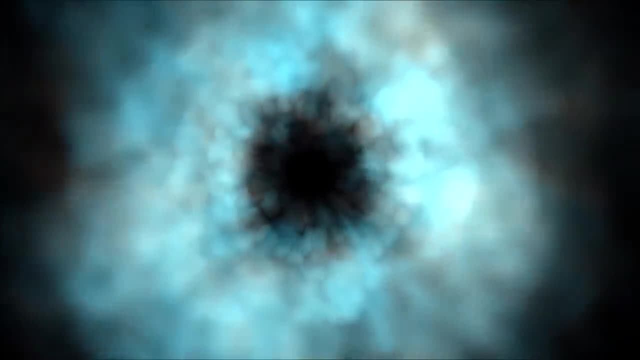 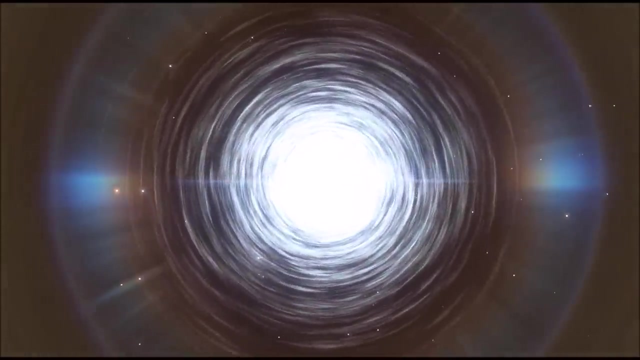 would be dispersed in every direction. Some of this matter falls straight into the black hole, whereas some of it may be ejected beyond the event horizon at immense speeds before falling back in again. Some of the debris will be flung out and will be under much less.